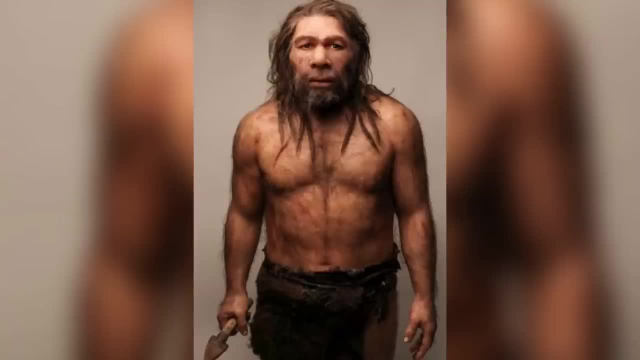 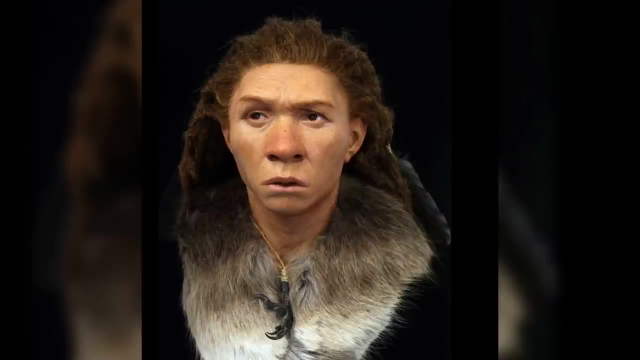 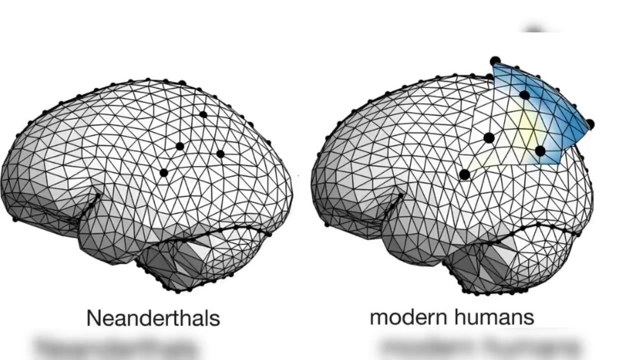 frame and strong limbs, adapted to the harsh climates they often inhabited. They had prominent brow ridges, wide noses and a unique forward-projecting mid-face. Their cranial capacity was, on average, slightly larger than that of modern humans, suggesting a large brain. 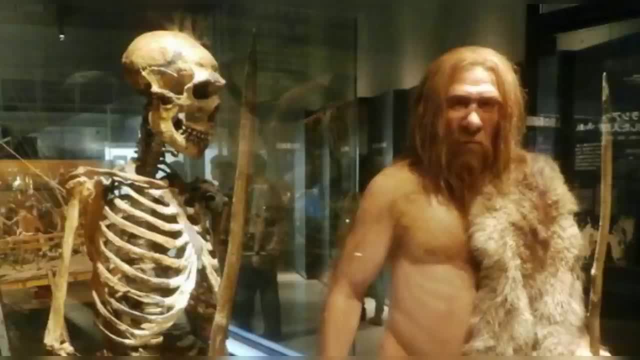 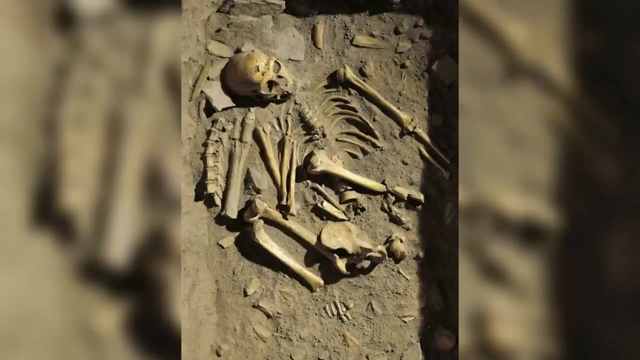 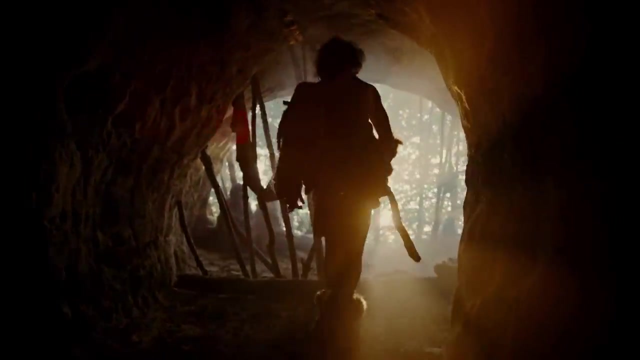 This physical build was likely an adaptation to cold environments, aiding in heat retention. The Neanderthals emerged approximately 400,000 years ago. based on fossil evidence, They thrived across Europe and parts of Asia during the Middle and Late Pleistocene Epoch. The most complete timeline of Neanderthal existence places them from about 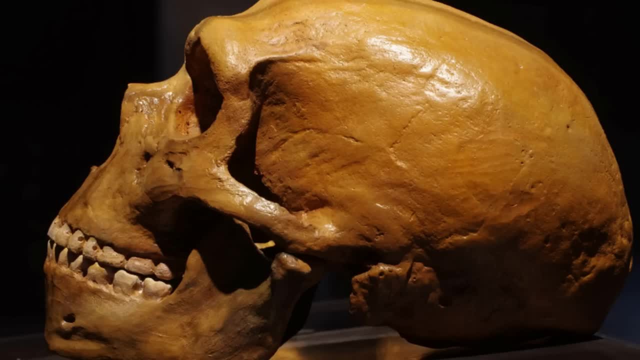 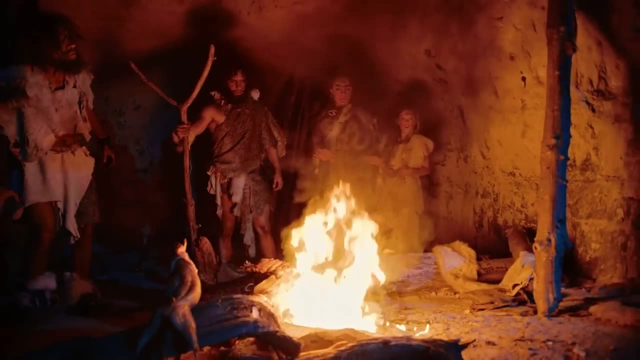 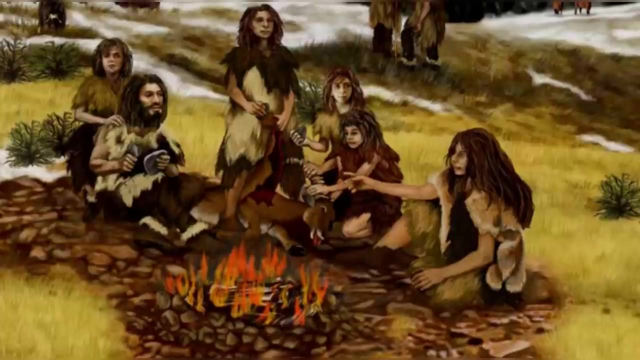 400,000 to 40,000 years ago. During this period, they experienced various ice ages and climate changes which significantly impacted their living conditions and survival strategies. Neanderthals were remarkably adaptable, surviving in a wide range of environments across their 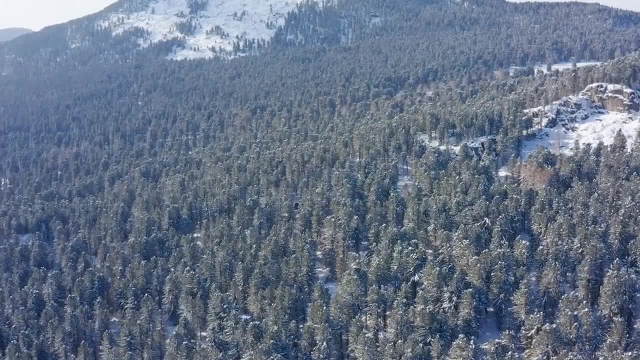 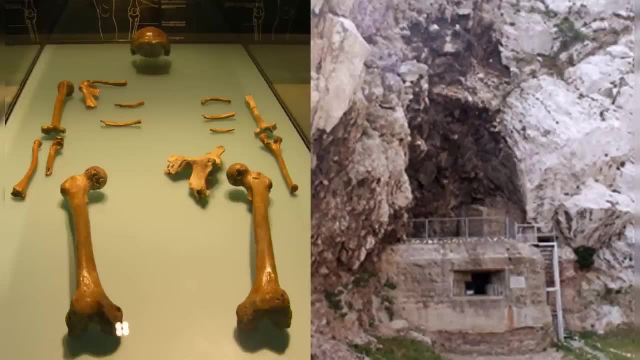 existence. They predominantly occupied regions in Europe, from Spain to Siberia, and extended into the Middle East. Notable sites include the Neander Valley in Germany, where the first recognized Neanderthal fossils were found, and other significant locations such as the caves of Atapuerca in Spain and Vindica Cave in Croatia. Their habitats varied from woodlands. 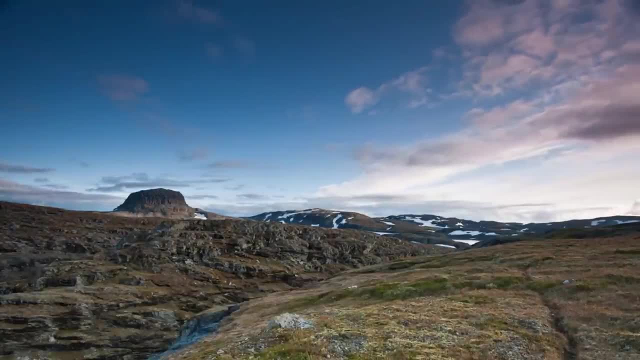 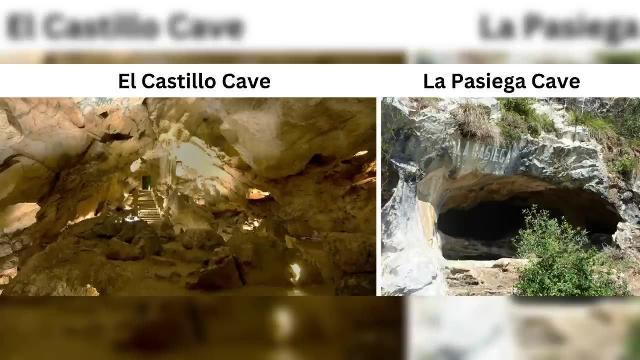 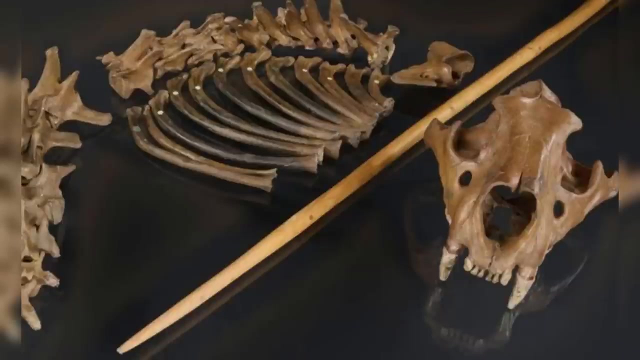 to steppes and even cold Arctic environments. They were capable of adapting to these diverse climates, as evident from their remains found in various ecological settings. Their adaptability is further underscored by the range of animal remains found near their sites, suggesting they could hunt a variety of prey. 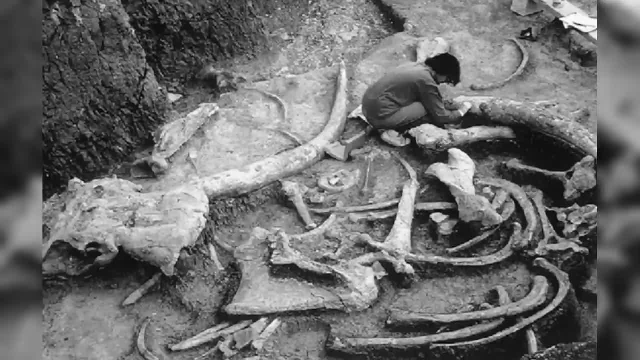 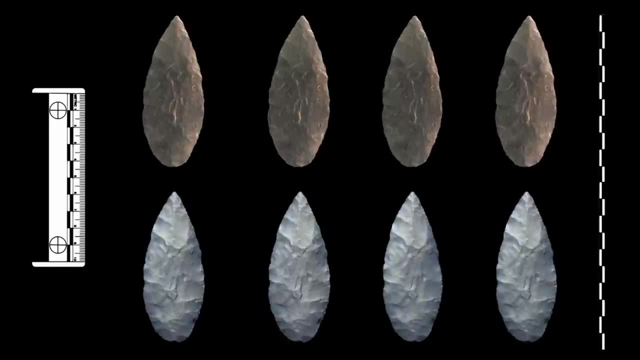 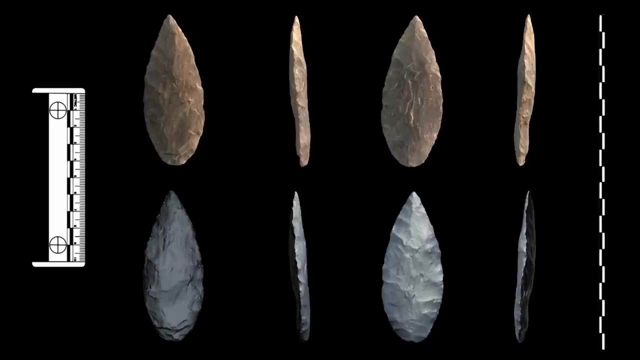 Neanderthals were skilled hunters capable of taking down large game such as woolly mammoths, bison and deer. Their tool technology, known as the Mysterian culture, was sophisticated and included a range of flint tools for hunting, butchering and scraping. Evidence also suggests: 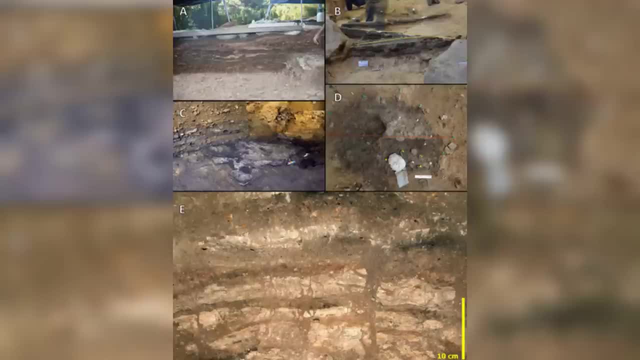 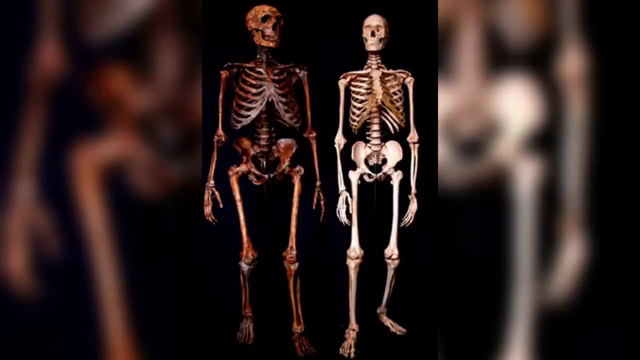 they used fire, constructed shelters and may have had some form of symbolic or ritualistic practices. One of the most intriguing aspects of Neanderthal history is their interaction with other human species, including Homo sapiens. Genetic evidence shows that there was interbreeding between 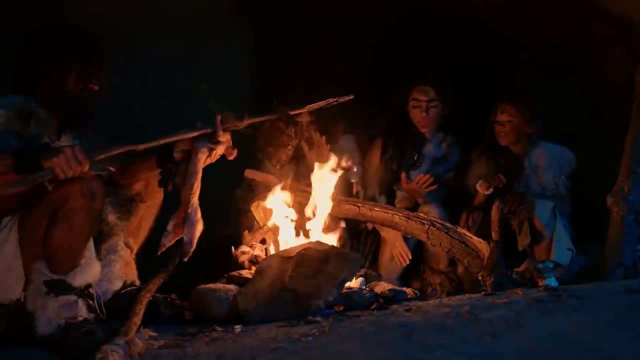 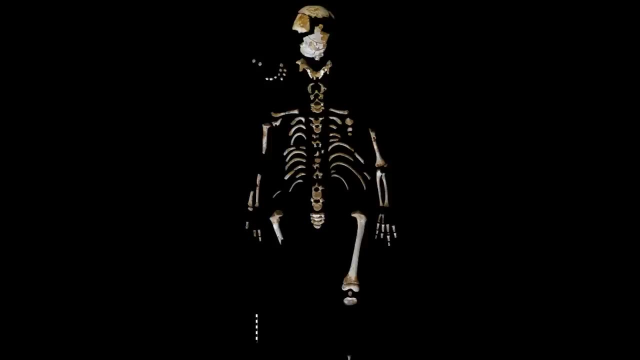 Neanderthals and modern humans, with non-African human populations today having about 1% to 2% Neanderthal DNA. The exact reasons for the Neanderthals' extinction around 40,000 years ago remain a subject of research. 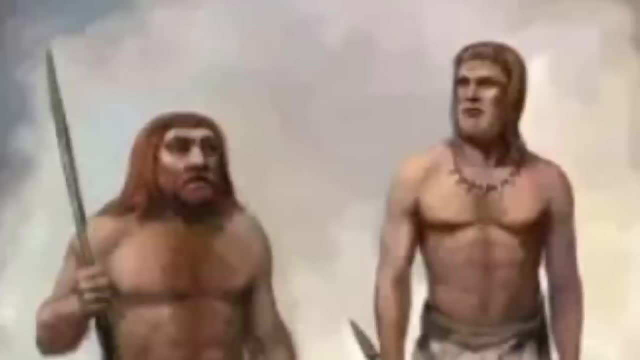 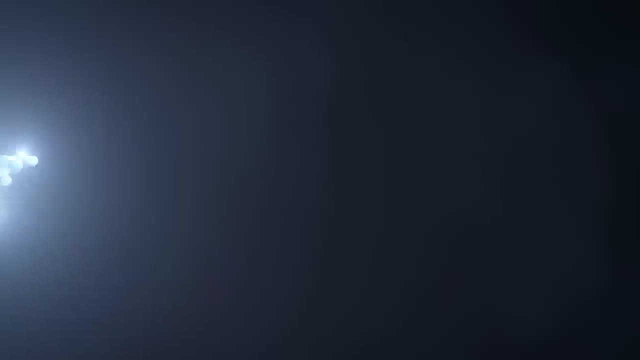 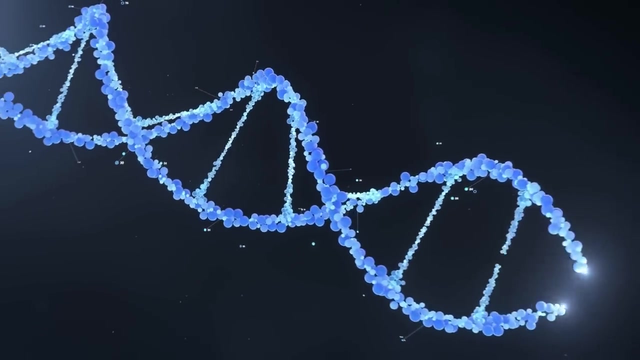 Hypotheses range from competition with Homo sapiens, climate change, a reduced capacity for adaptation to pandemics. However, their genetic legacy lives on in modern humans, providing a fascinating insight into our past. Understanding Neanderthals offers a window. 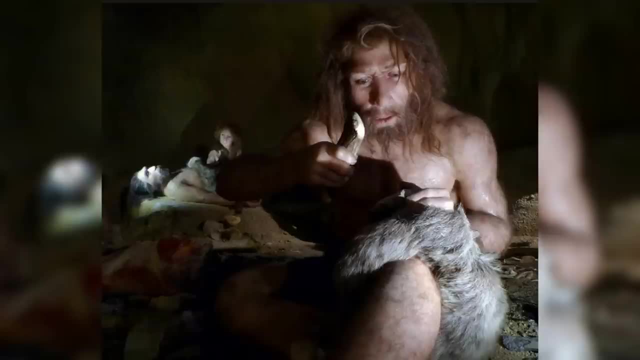 into a critical period of human history. They were not the brutish primitive beings as once thought, but a resilient, agile and resilient human race. Neanderthals were a versatile, adaptable species that survived challenging environmental changes and left a lasting impact on the human genetic blueprint. 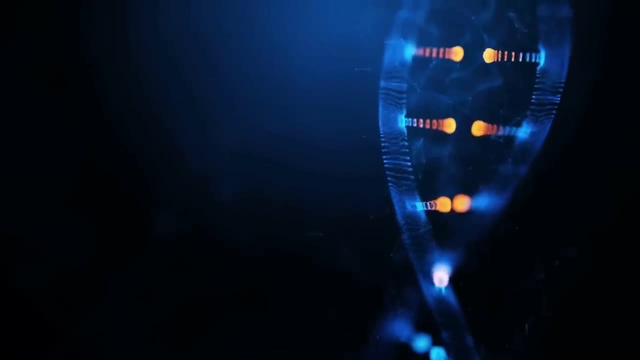 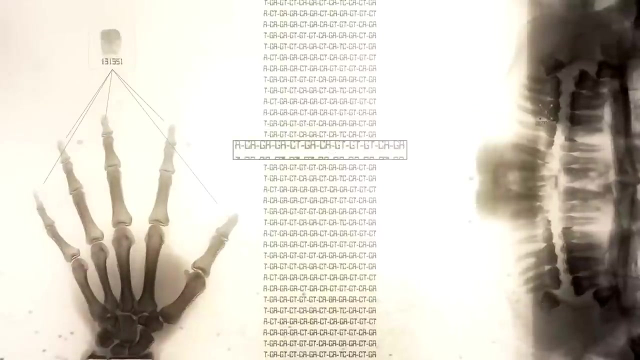 The discovery that modern humans carry Neanderthal genes was a groundbreaking development in the field of genetics and human history. This revelation came to light with the advent of advanced DNA sequencing technologies. In 2010,, a significant study published by the Max Planck Institute published in the late 1970s, came to light. The providence of advanced DNA sequencing technologies arrived to the attention of the world in 2010.. The last scientific research carried out on the Neanderthal gene was the focus of the human genome, even more so that 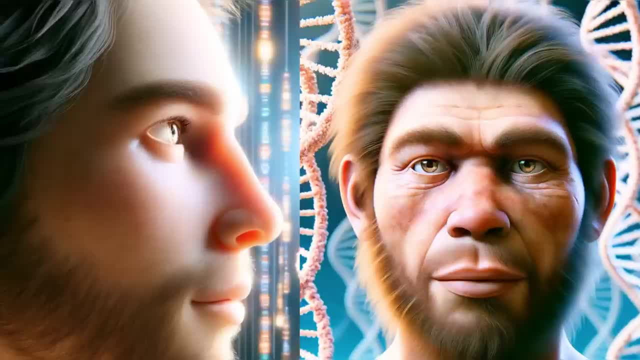 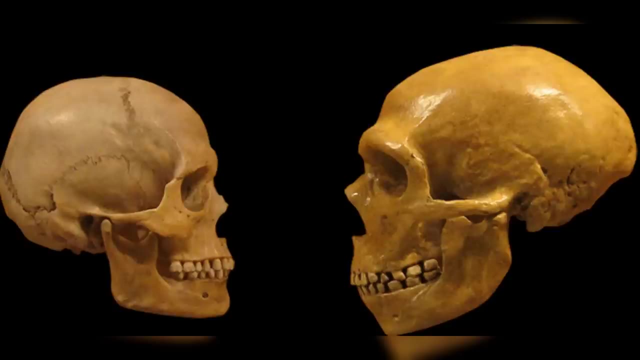 Institute in Leipzig, Germany, revealed that between 1% and 2% of the genome of people with Eurasian ancestry can be traced back to Neanderthals. The presence of Neanderthal DNA in modern humans is attributed to interbreeding between 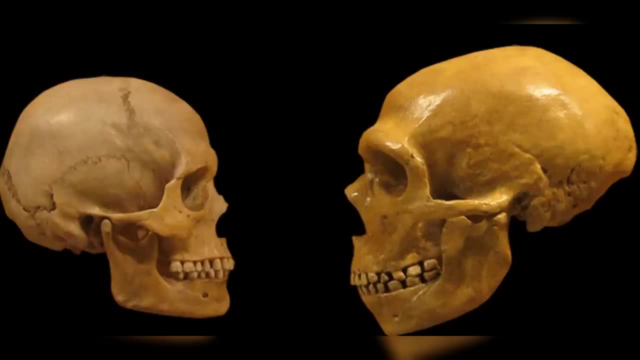 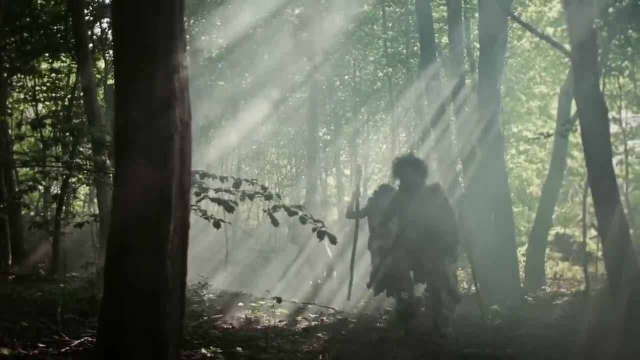 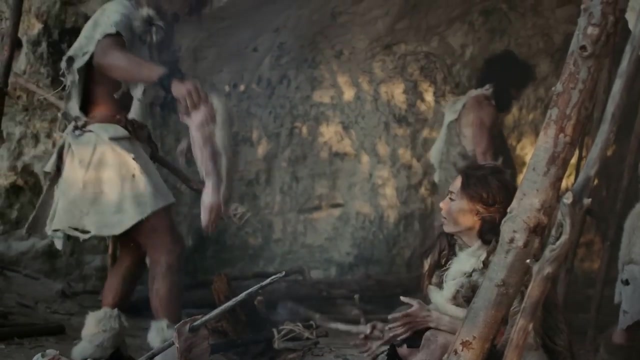 Neanderthals and anatomically modern Homo sapiens. This interbreeding likely occurred 50,000 to 60,000 years ago, when modern humans encountered Neanderthals in Europe and Asia. The genetic exchange suggests that Neanderthals and modern humans were closely related enough. 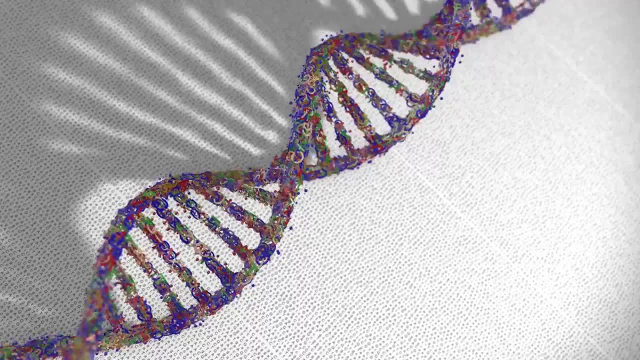 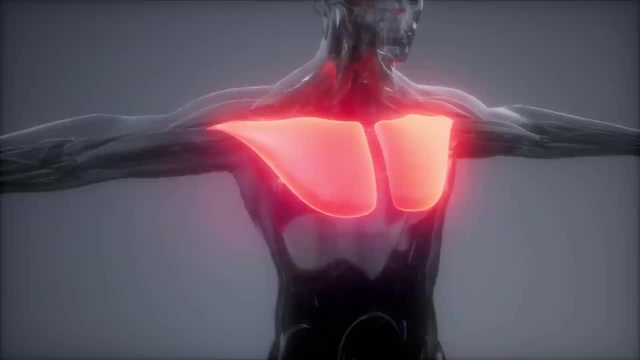 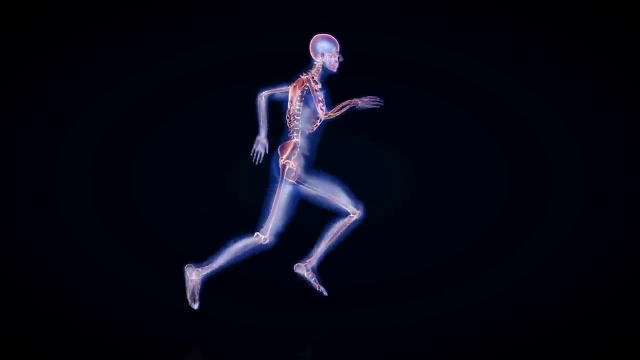 to produce fertile offspring. The proportion of Neanderthal DNA varies among different human populations. The Neanderthal genetic contribution has been linked to various genetic contributions. There are various aspects of human biology. Some of these genes are believed to have offered adaptive advantages to early modern humans. 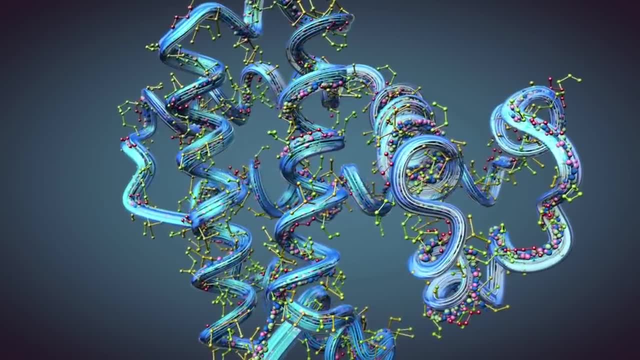 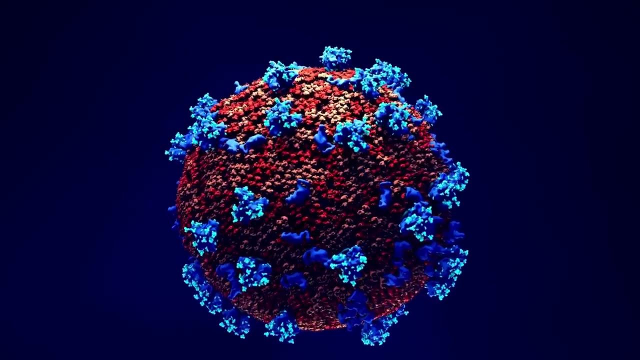 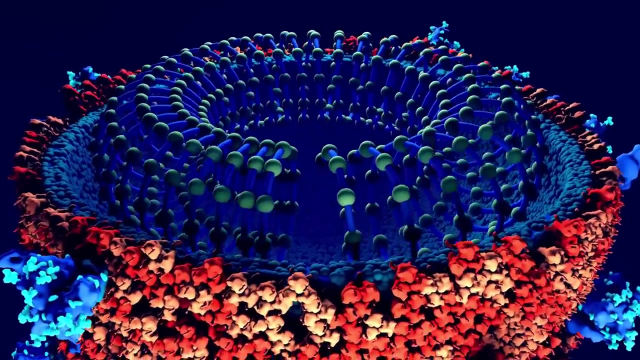 For instance, there are genes related to keratin protein which may have helped humans develop tougher skin, better suited to colder climates. Other genes are associated with hair and skin color variation, immune system function and even the risk of developing certain diseases. 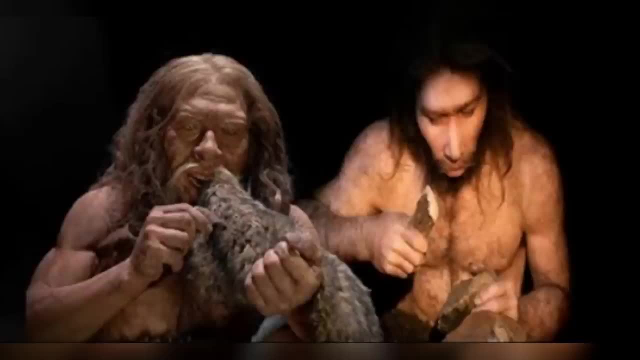 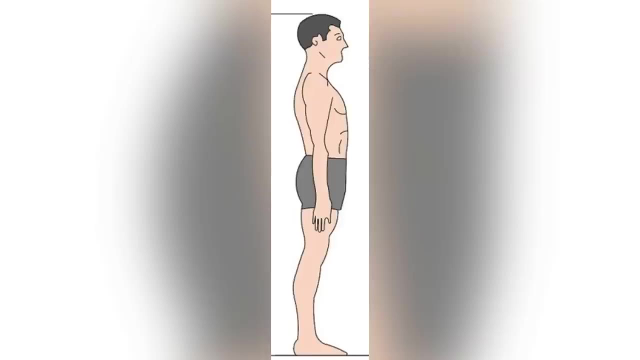 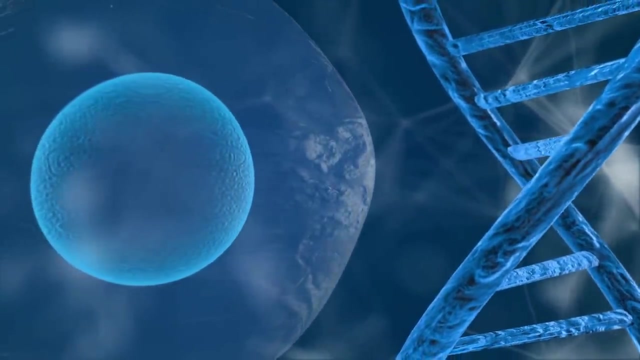 Ongoing research continues. Using genetic data can be used to uncover the influences of Neanderthal genes. Certain traits like height and sleeping patterns have also been linked to Neanderthal ancestry. The process through which modern humans inherited Neanderthal genes is complex. 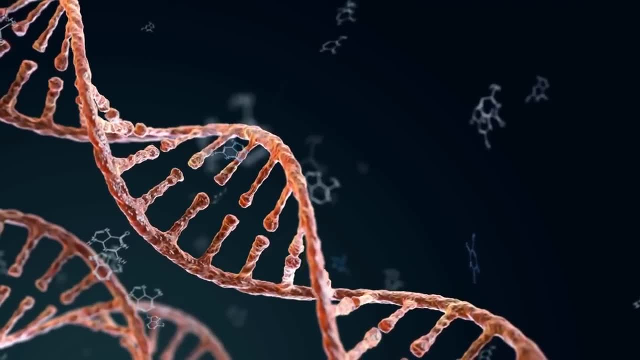 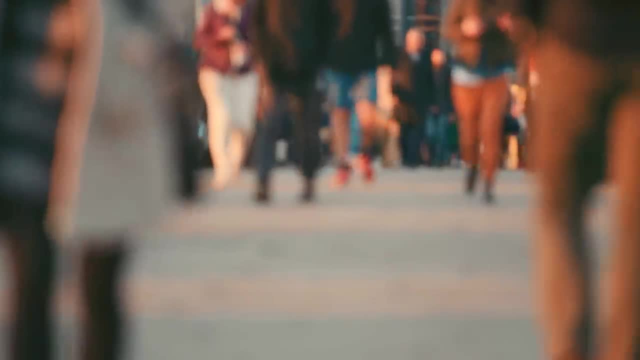 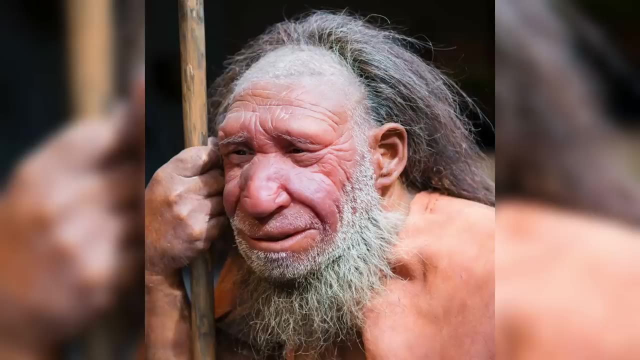 While some Neanderthal genes have been retained through positive selection, others have diminished over time due to genetic drift or negative selection- varied distribution of these ancient genes in different human populations. The discovery of Neanderthal DNA in modern humans has provided profound insights into 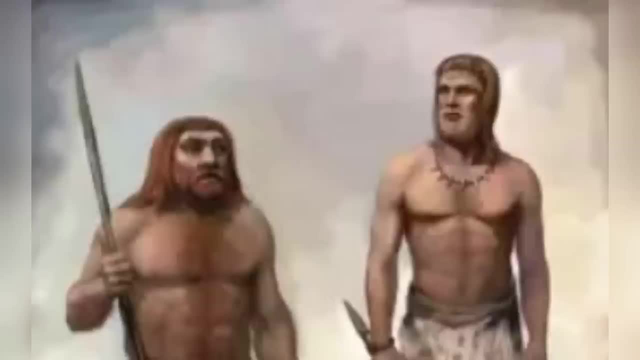 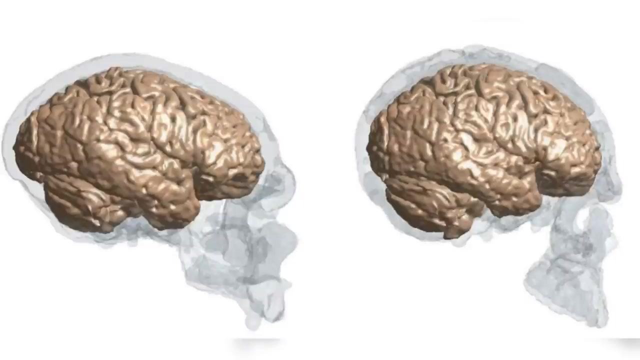 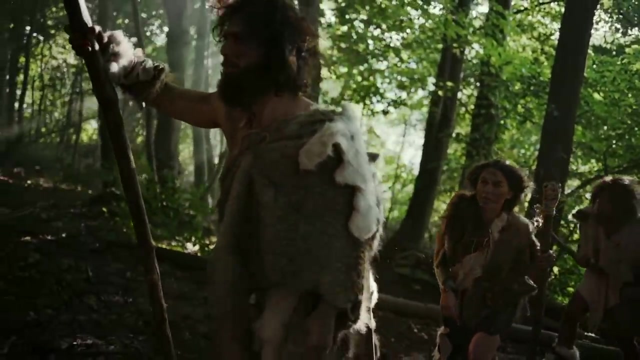 our past. It challenges previous notions of distinct species separations and highlights a more intertwined human history. This genetic inheritance is not just a relic of the past, but continues to influence the biological and possibly behavioral aspects of human life today. These insights into the relationship between modern human DNA and Neanderthal genes offer 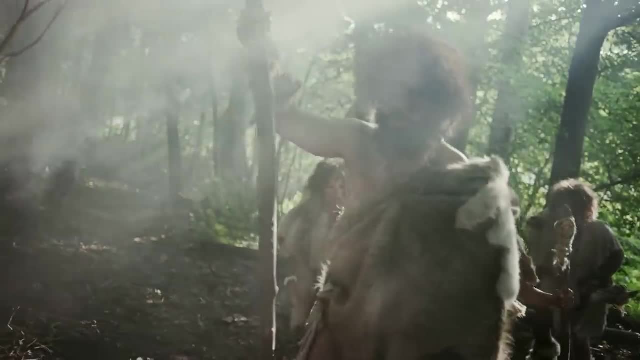 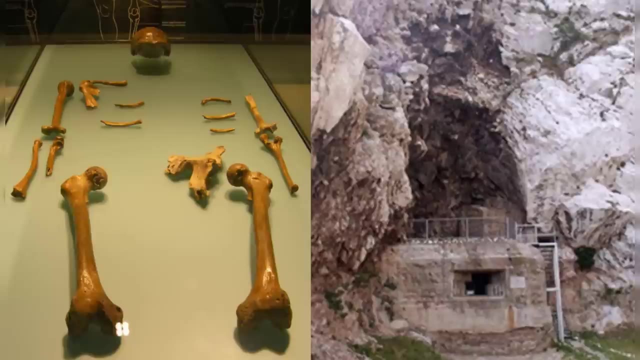 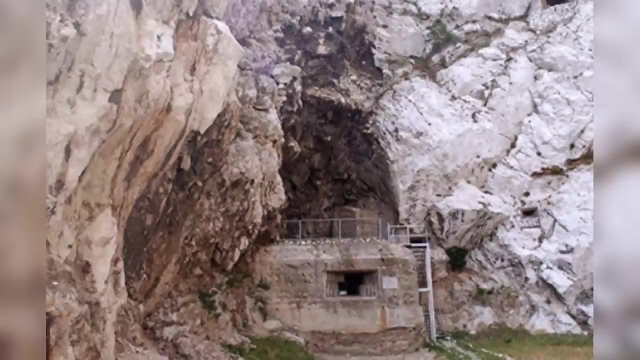 a fascinating glimpse into our shared history, adding depth to our understanding of human origins and diversity. The first recognized discovery of Neanderthal fossils dates back to 1856 in the Neander Valley near Dusseldorf, Germany. This site, a limestone quarry in the Feldhofer Cave, was where quarry workers unearthed a. 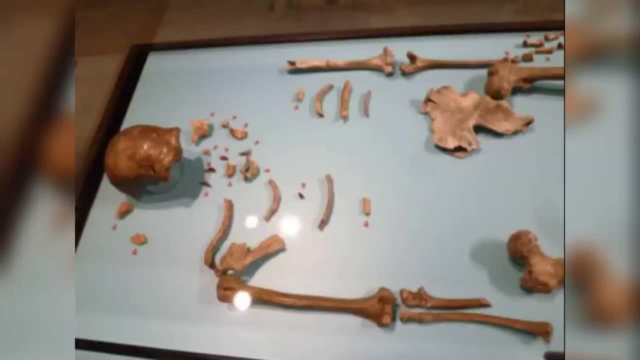 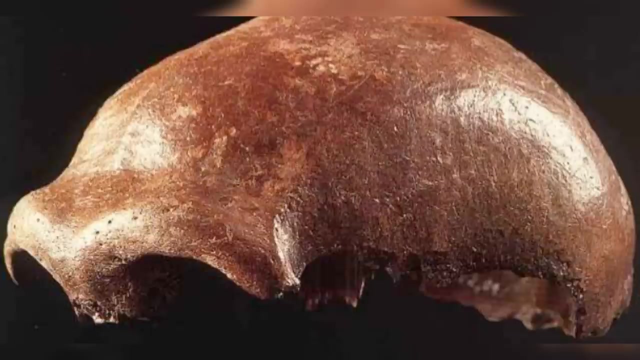 set of unusual bones. These included a skullcap, ribs, a part of a pelvis and limb bones which exhibited distinct characteristics not typical of modern humans. The bones were characterized by a low, elongated skull, thick brow ridges and a lack of a. 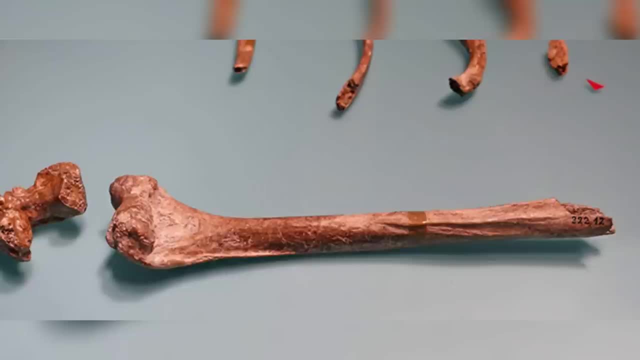 chin. Initially, the significance of these findings was not found. The bones were found in the Neanderthal's skull, which is the most important part of the Neanderthal gene. The bones were not fully understood and there was skepticism in the scientific community. 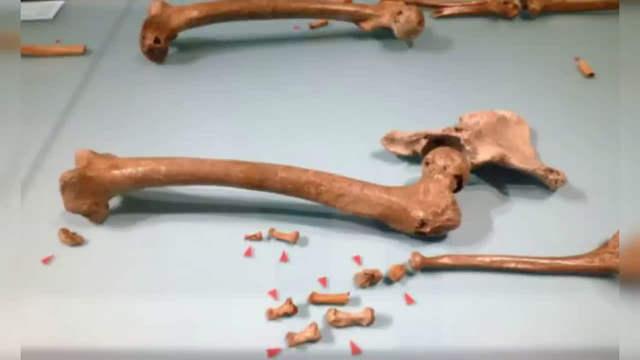 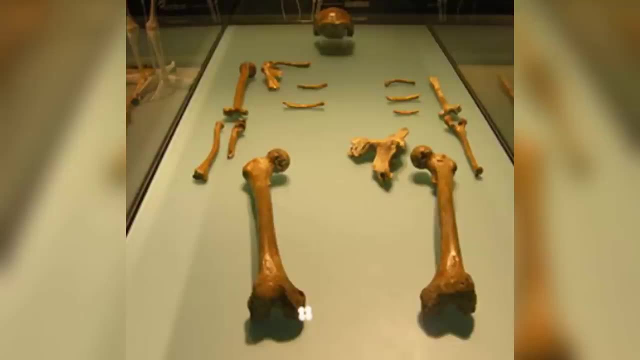 Some scientists of the time speculated that the bones might belong to a modern human with pathological conditions. It wasn't until years later, as more fossils were discovered, that the scientific community began to recognize these as belonging to a different human species. Following the initial discovery, numerous other Neanderthal fossils were found in various 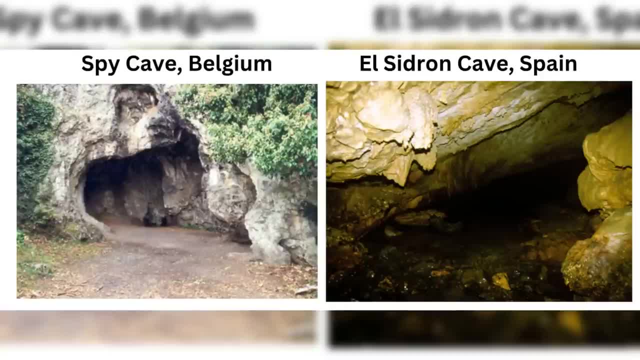 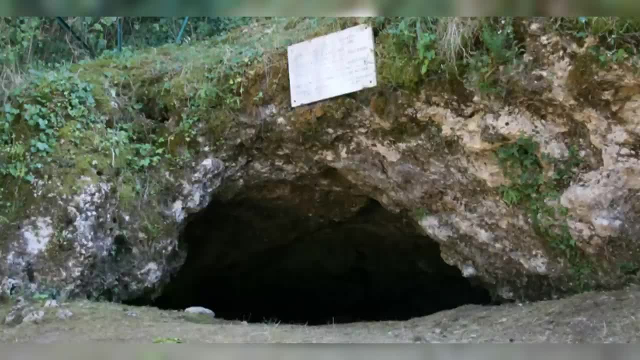 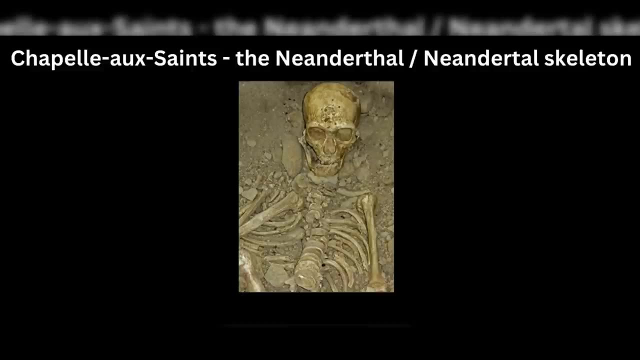 parts of Europe. Some of them were found in Europe and Western Asia, significantly contributing to our understanding of this species. Some notable sites included La Chapelle-aux-Seins, France, in 1908.. La Chapelle-aux-Seins provided one of the most complete Neanderthal skeletons, which 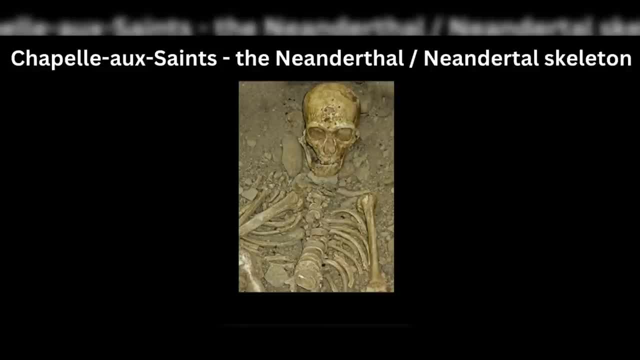 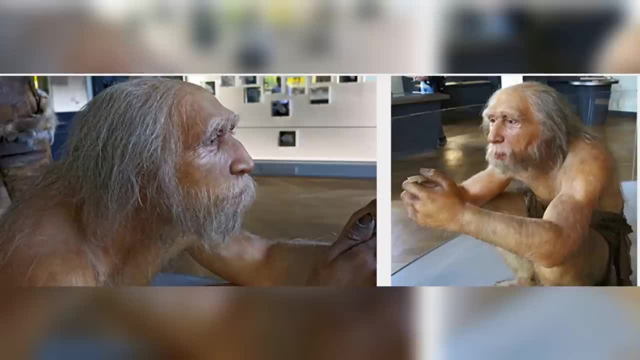 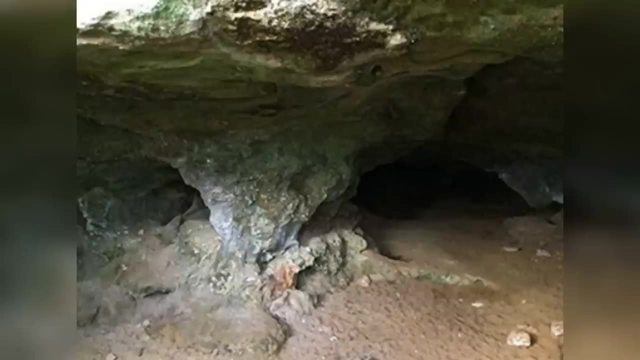 fueled the stereotype of Neanderthals as brutish and stooped. This interpretation was later revised as the individual was found to have suffered, hopefully, from severe arthritis. Le Moustier, in France, known for the discovery of a Neanderthal child and for giving its 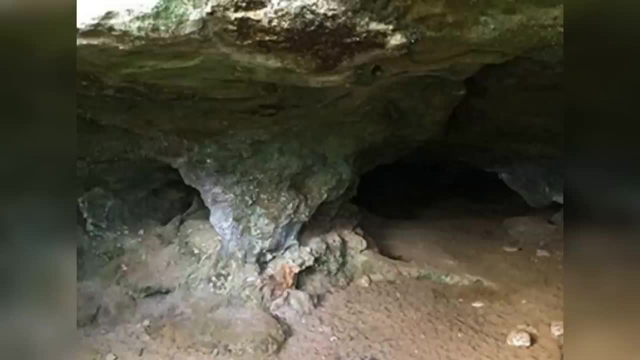 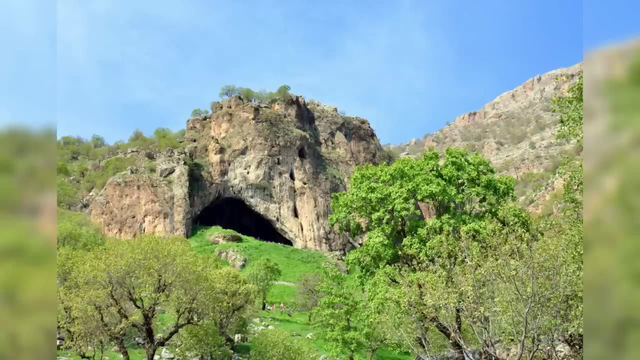 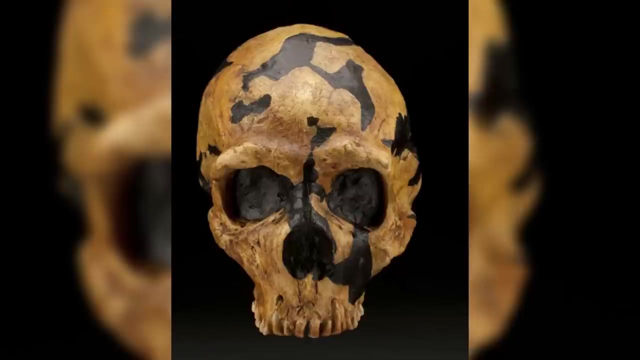 name to the Mousterian tool culture associated with Neanderthals. Shanidar Cave in Iraq. the site yielded several Neanderthal skeletons. The discovery of pollen around one of the skeletons known as Shanidar IV led to speculation about burial rituals and the potential for Neanderthal concepts of Neanderthalritic. 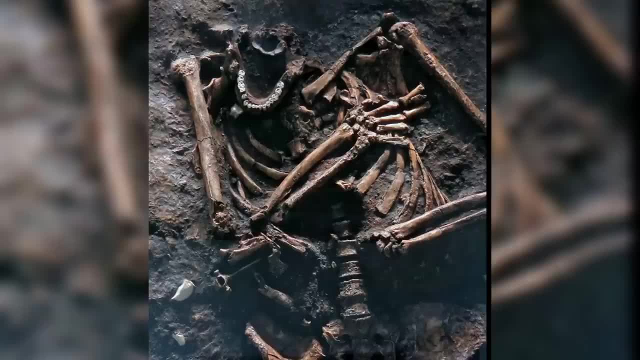 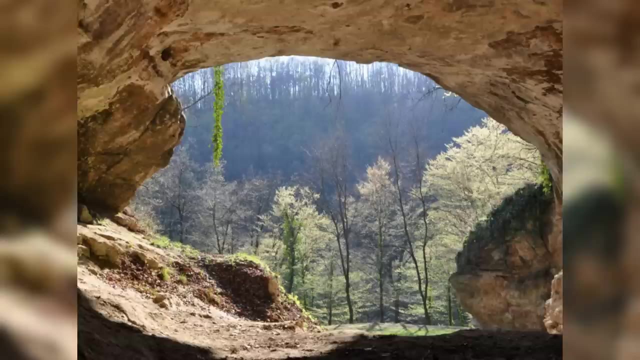 of the afterlife. Kabara Cave in Israel. the discovery of a nearly complete Neanderthal skeleton here, especially the hyoid bone, contributed significantly to discussions about Neanderthal speech capabilities. Vindija Cave in Croatia, here late surviving Neanderthal. 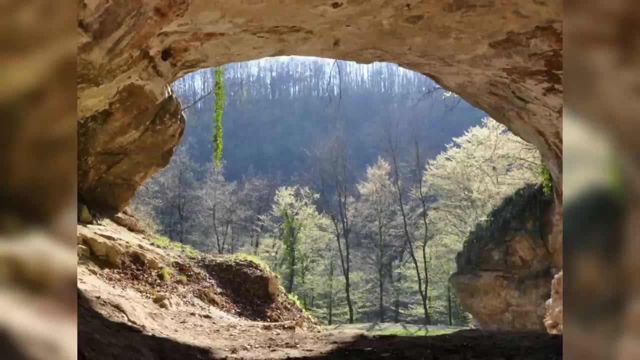 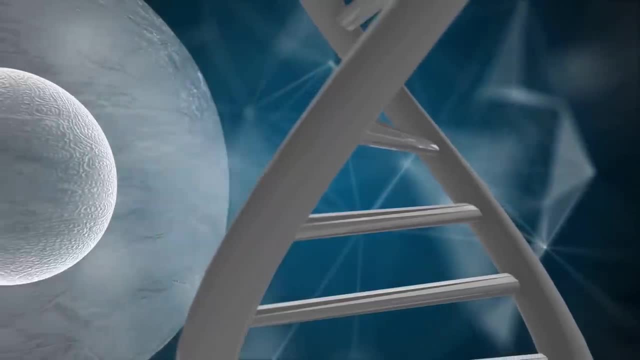 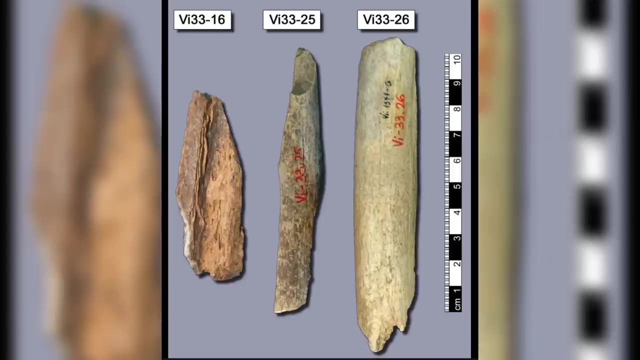 remnants were found, pushing back the timeline of Neanderthal extinction and indicating potential overlap and interaction with modern humans. Advances in genetic techniques in the 21st century have been pivotal in understanding Neanderthals. The sequencing of the Neanderthal genome from fossils, especially those from Vindija Cave, allowed scientists to compare it. 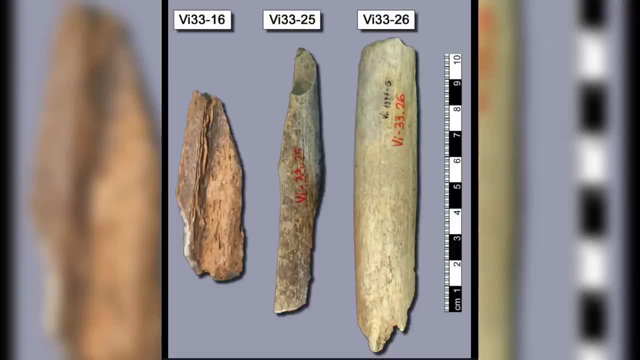 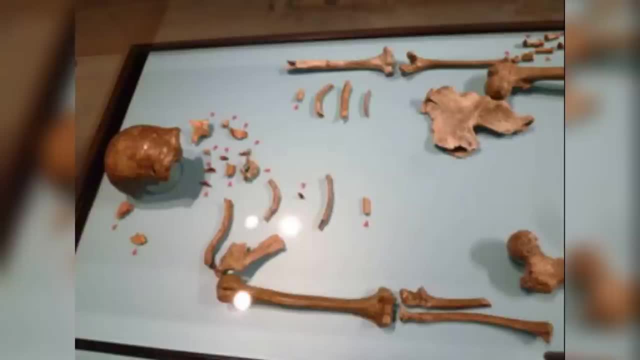 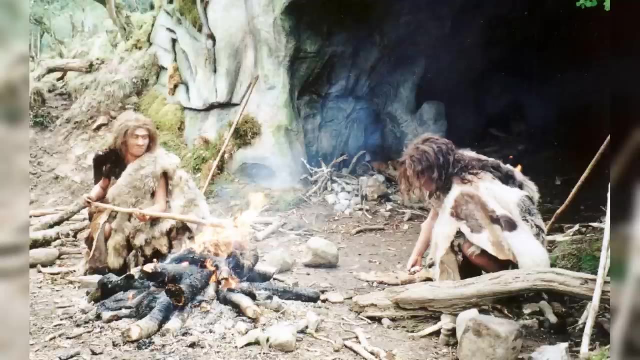 with modern human DNA, revealing interbreeding and genetic exchange. The discovery of Neanderthal fossils beginning in the Neander Valley was pivotal in shaping our understanding of human history. Each subsequent discovery added layers of complexity to our understanding of Neanderthals from their physical characteristics and cultural practices. 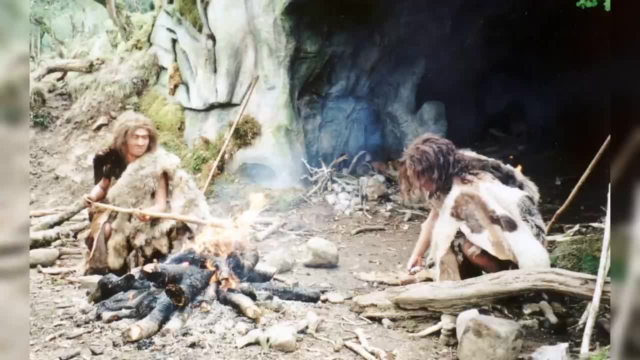 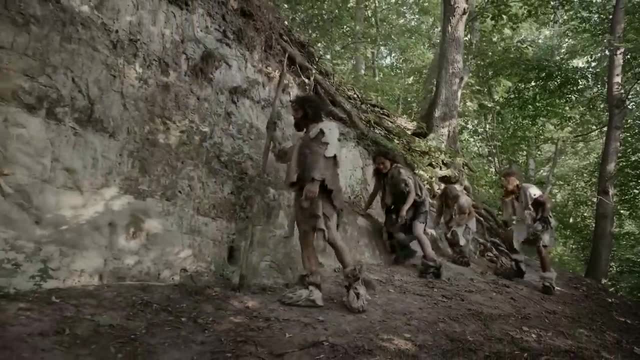 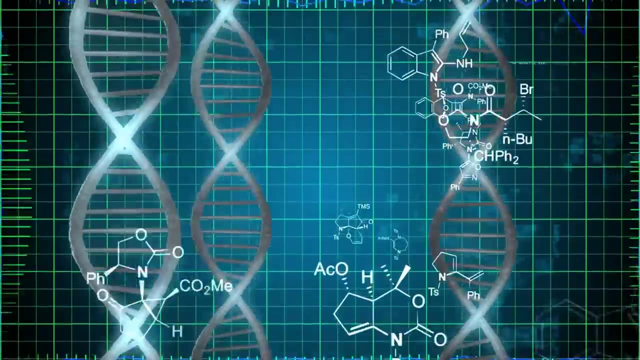 to their genetic contribution to modern humans. These findings, spread across various sites in Europe and Asia, offer invaluable insights into a species that once walked the earth alongside our ancestors. The development of DNA analysis, culminating in the ability to sequence the Neanderthal genome. 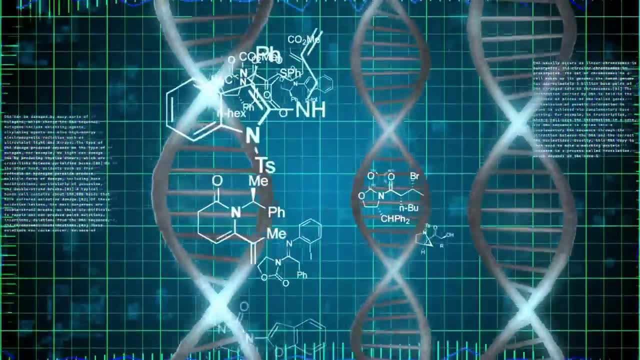 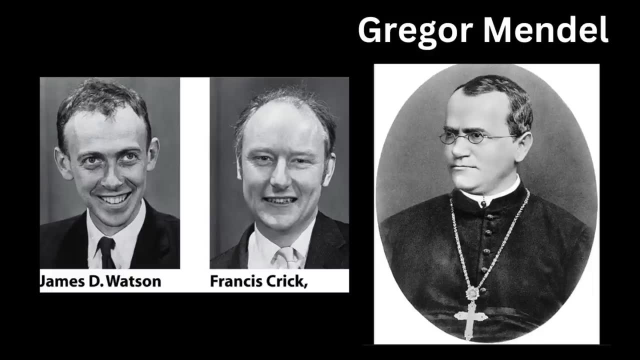 represents a remarkable journey in the field of genetics and paleoanthropology. The journey began with the foundational work in genetics by scientists like Gregor Mendel in the 19th century and the discovery of the DNA double helix structure by Watson and Crick in 1953. 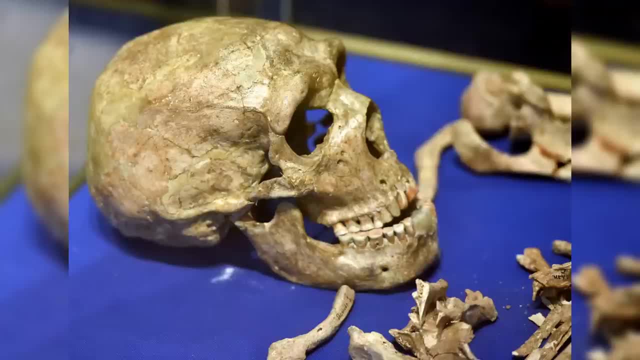 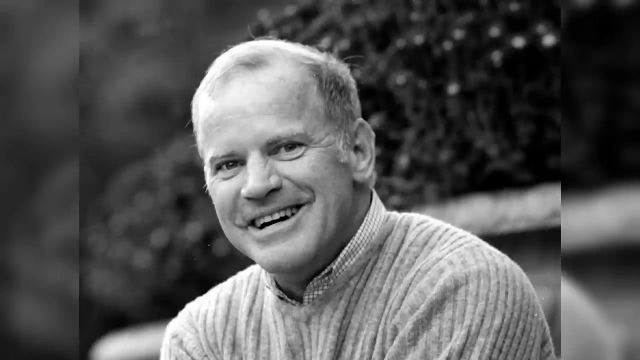 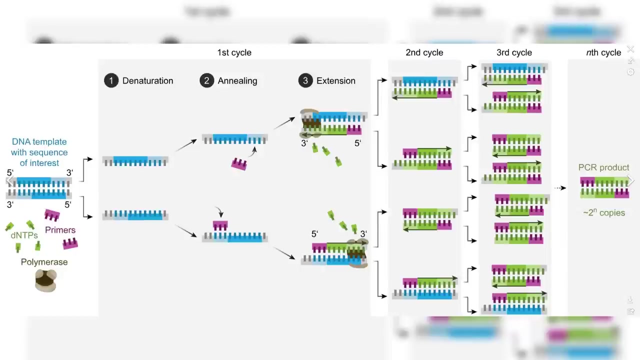 However, the ability to analyze ancient DNA from fossils took much longer to develop due to technical challenges such as contamination and degradation of DNA over time. A significant breakthrough came with the invention of the polymerase chain reaction, or PCR, in the 1980s by Carey Mullis. PCR allowed scientists to amplify 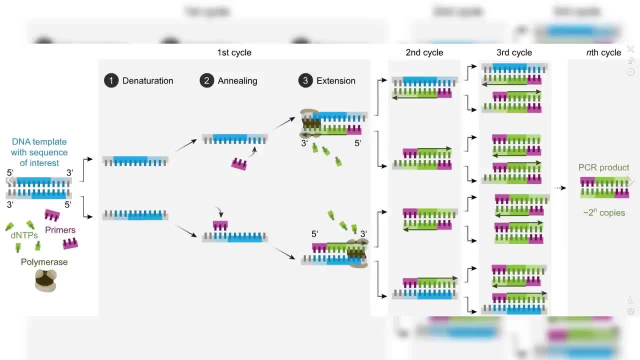 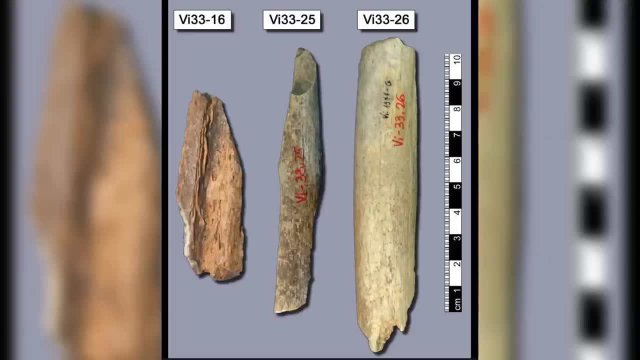 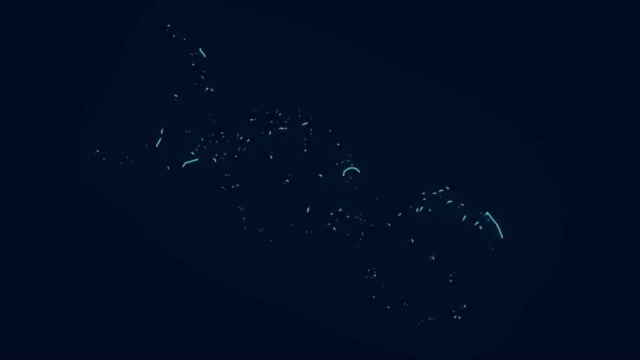 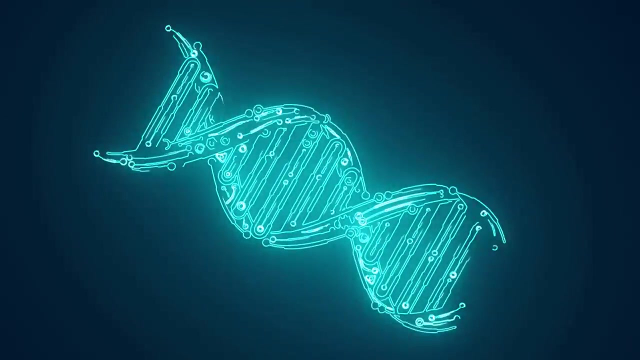 small segments of DNA, making it possible to study genetic material even from ancient specimens. This technology was crucial in the early attempts to extract and amplify DNA from Neanderthal fossils. The advent of next-generation sequencing technologies in the early 21st century dramatically changed the landscape of genetic research. These technologies 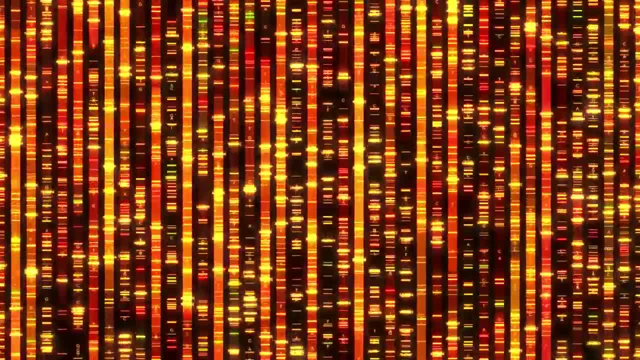 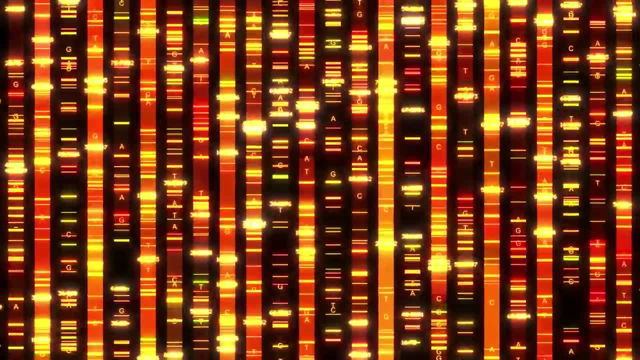 such as those developed by companies like Illumina and 454 Life Sciences, enabled the sequencing of entire genomes quickly and quickly. The technology was used in the early 20th century to detect and, and, more affordably, It became feasible to contemplate sequencing ancient genomes. 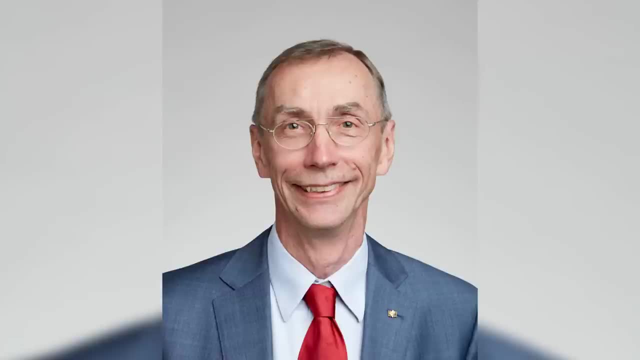 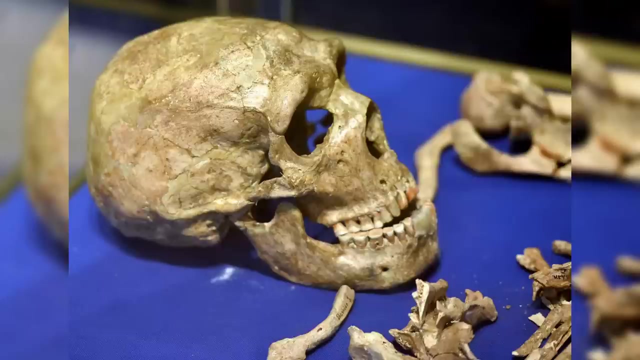 including that of Neanderthals. The Neanderthal Genome Project, initiated in 2006,, was a landmark effort led by Svante Paebo at the Max Planck Institute for Evolutionary Anthropology. This project aimed to sequence the entire Neanderthal genome. The team faced numerous 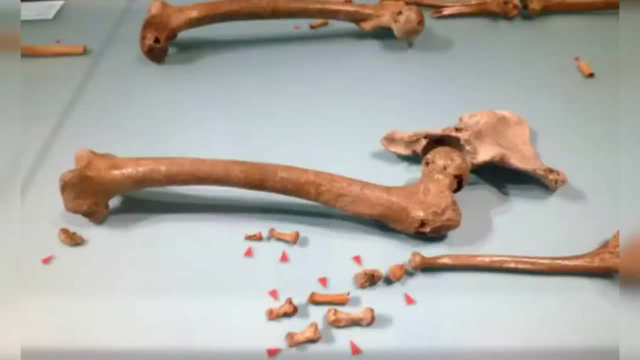 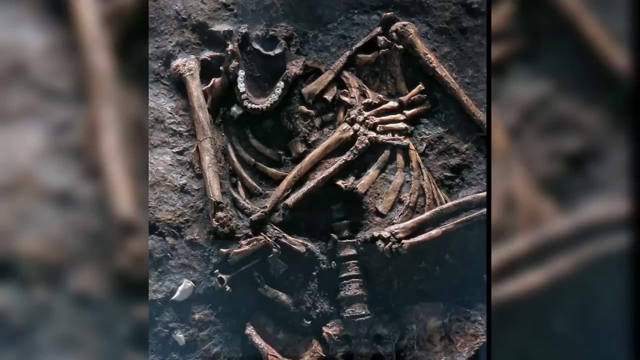 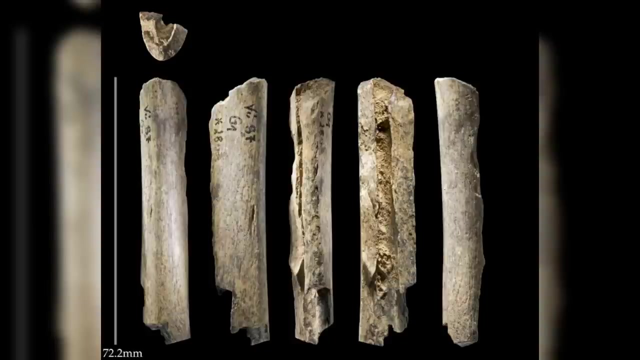 challenges, including contamination with modern human DNA and the degradation of the Neanderthal DNA over tens of thousands of years. The key to success was meticulous sample selection and contamination control. The team used bone fragments from several Neanderthal individuals, with major contributions coming from specimens found in Vindia Cave, Croatia. 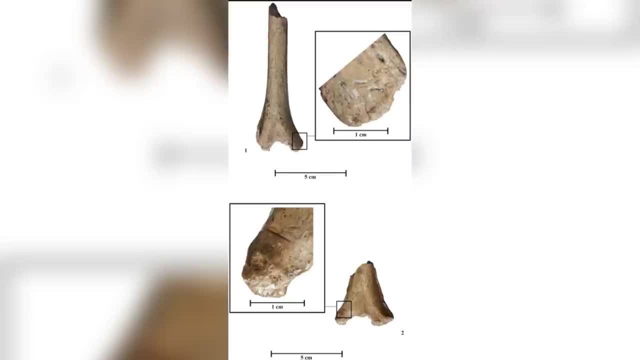 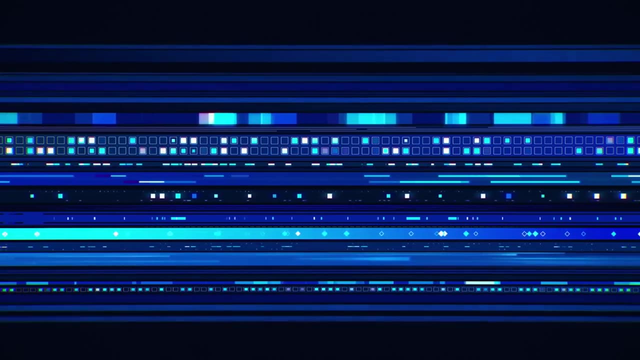 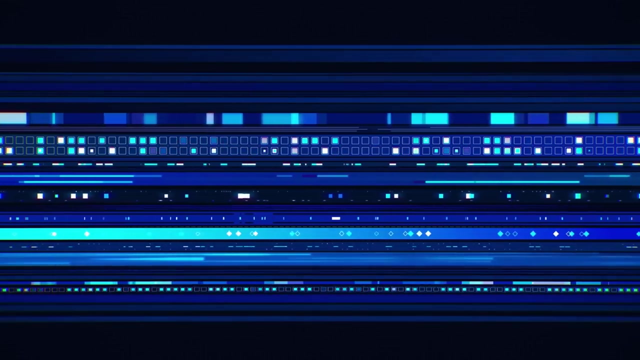 These samples were less contaminated and better preserved, providing high-quality genetic material for sequencing. Using advanced sequencing techniques, the team managed to extract, sequence and piece together the Neanderthal genome from these tiny bone fragments. They compared this genome with those of modern humans and identified segments of Neanderthal. 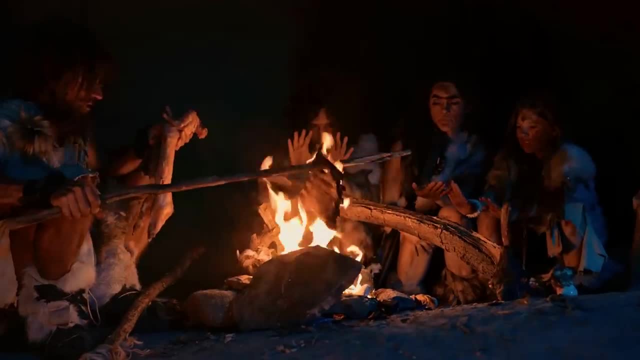 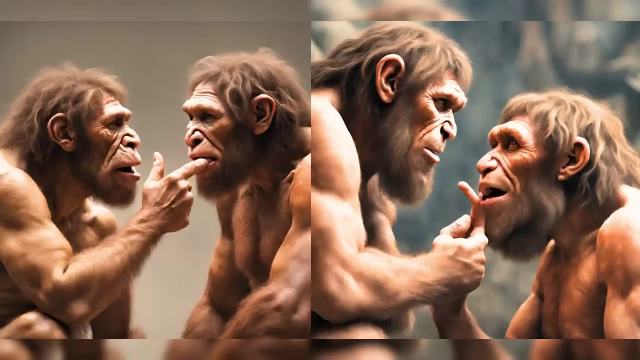 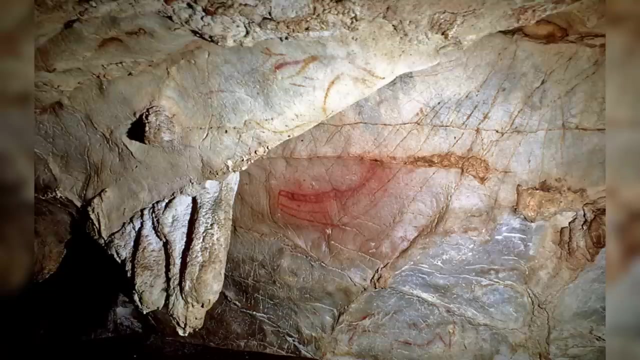 origin in the DNA of contemporary non-African populations, confirming interbreeding between Neanderthals and early modern humans. The successful sequencing of the Neanderthal genome was a watershed moment. It not only proved that Neanderthals contributed to the genetic makeup of modern humans, but also opened new 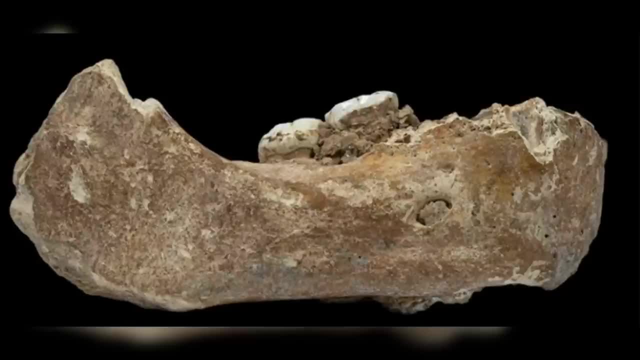 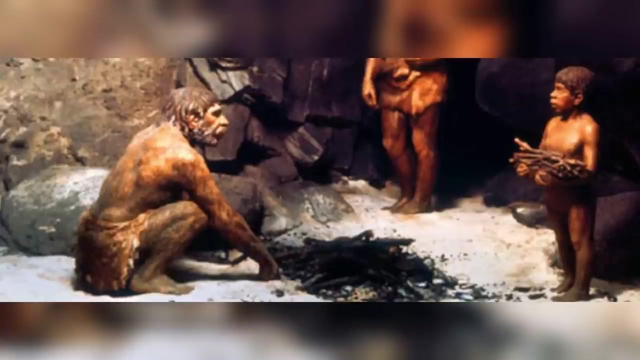 avenues for understanding human history. This achievement paved the way for further studies, including the sequencing of other ancient human genomes, like that of the Denisovans, another extinct hominin species. This endeavor has provided unprecedented insights into our past, reshaping our understanding of 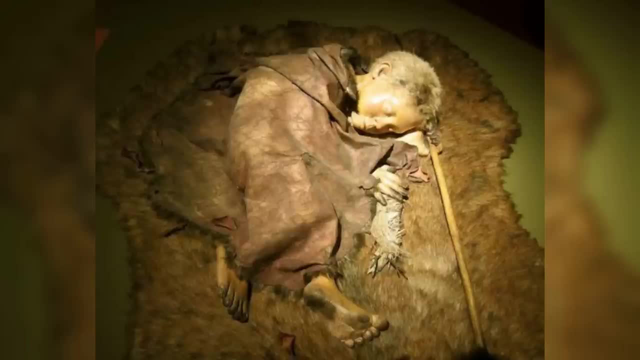 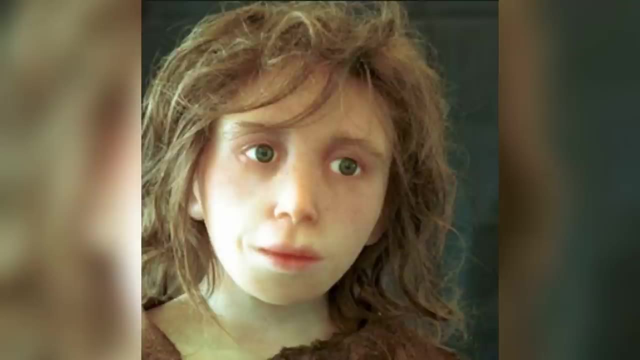 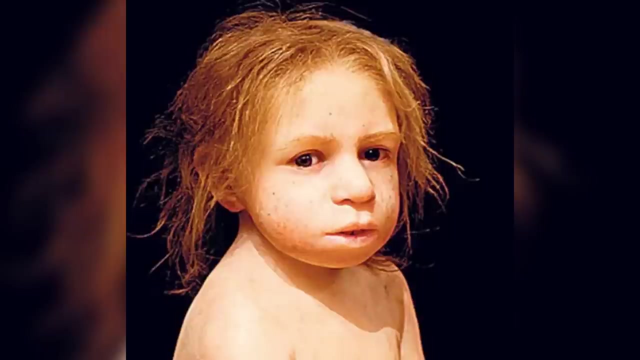 human history. There are many key aspects to this newfound ability. Traditionally, human history was often viewed as a linear progression from primitive to more advanced forms, culminating in modern Homo sapiens. The revelation of interbreeding between Neanderthals. 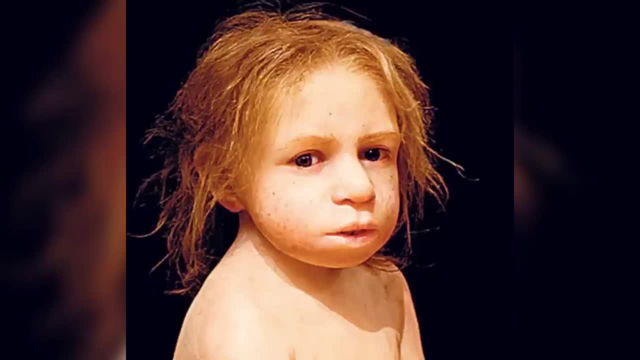 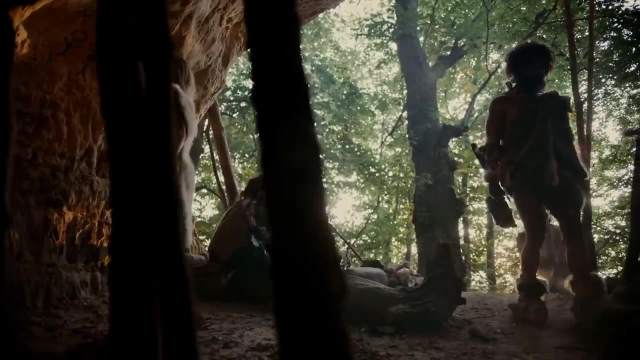 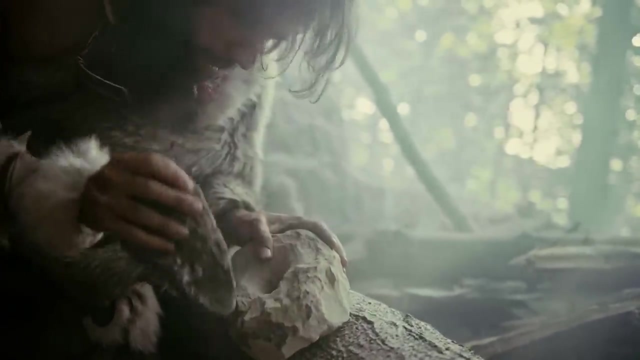 and Homo sapiens disrupted this linear narrative. It suggested a more complex web of interactions and genetic exchange between different hominin species. This has led to a more nuanced understanding that human history is not a straight line but a branching tree with many interconnected paths. 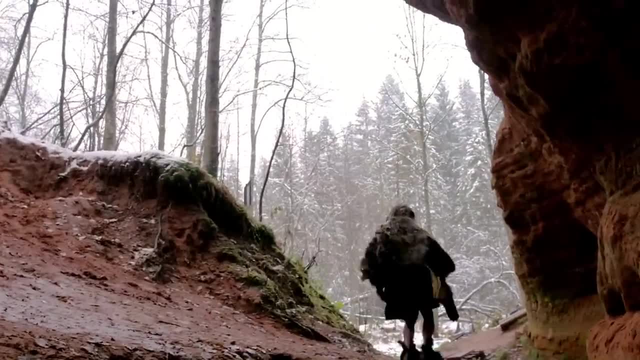 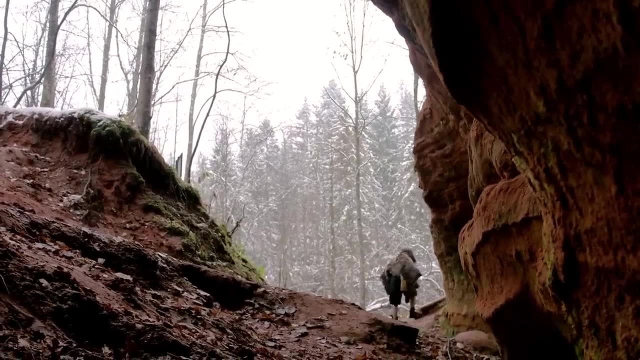 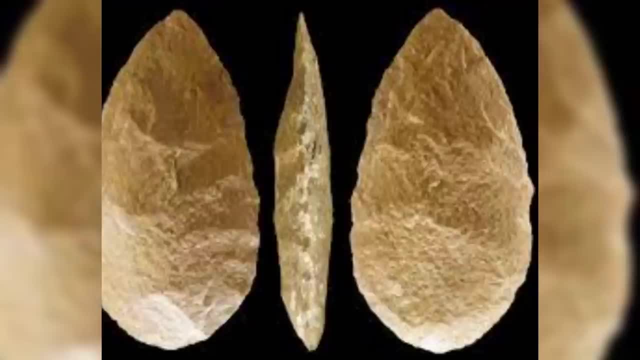 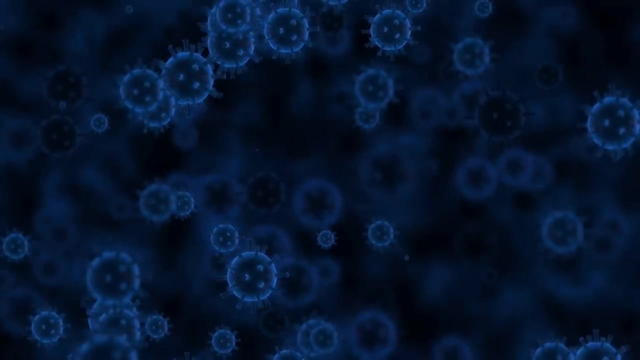 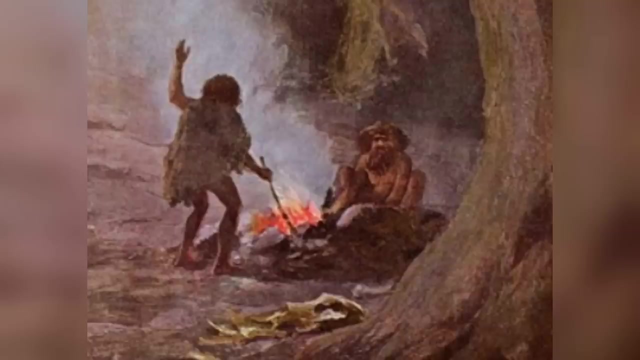 studies on tool-making techniques and cultural artefacts from sites across Europe provide insights into these differences in innovation and adaptability. The interaction between Neanderthals and modern humans could have facilitated the transmission of pathogens. Modern humans might have carried diseases to which Neanderthals had no immunity. 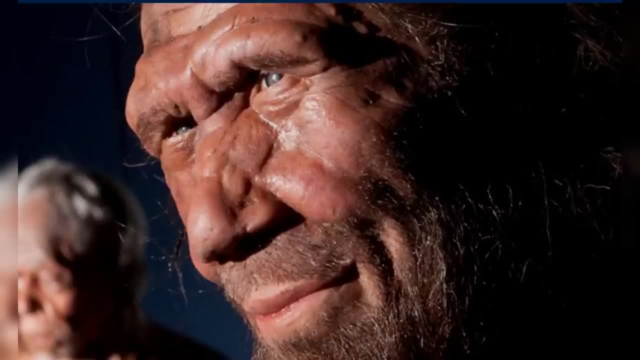 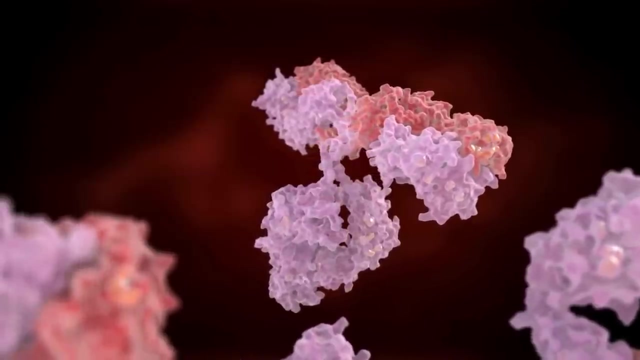 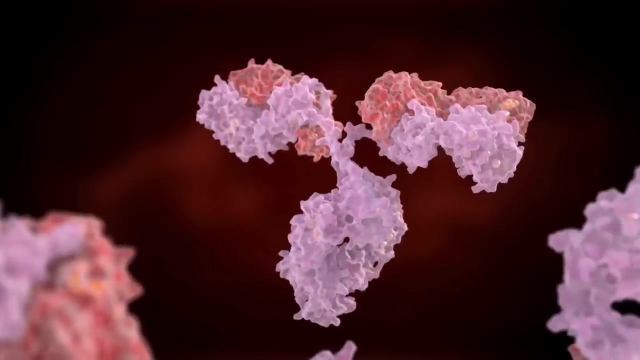 This theory, explored in research from institutions like the University of Oxford, suggests that disease transmission could have contributed significantly to the decline in Neanderthal populations. Genetic studies indicate that while some Neanderthal genes boosted the immune system of modern humans, the hybrid offspring might have had complex immune responses. 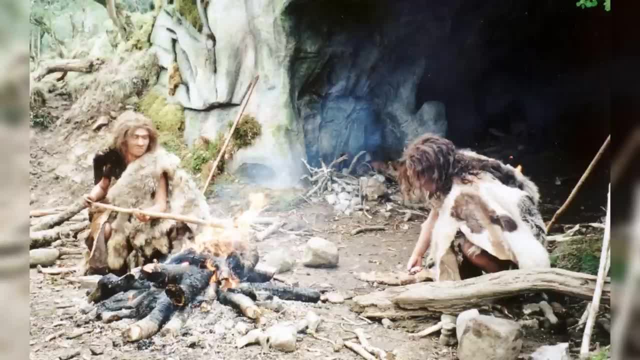 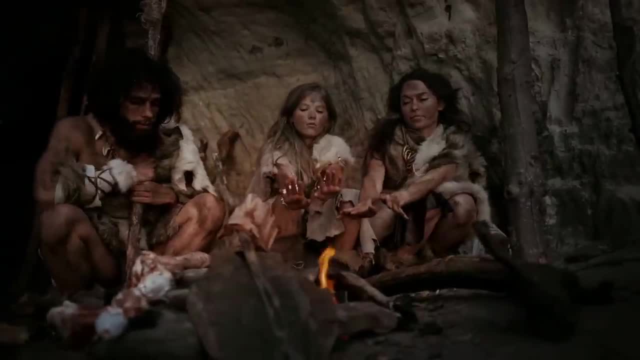 This could have made them more susceptible to some of the most common diseases of the human body. There are certain diseases affecting the health and longevity of the Neanderthal population. The extinction of Neanderthals is likely the result of a combination of factors. 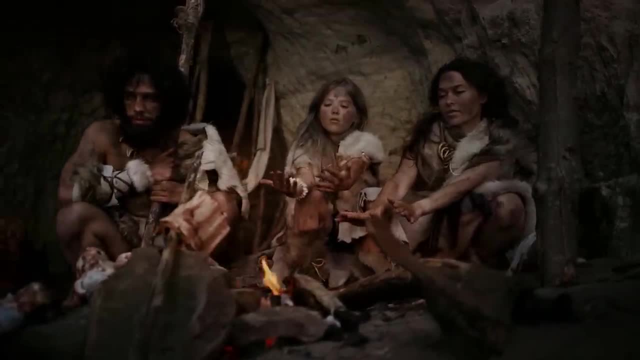 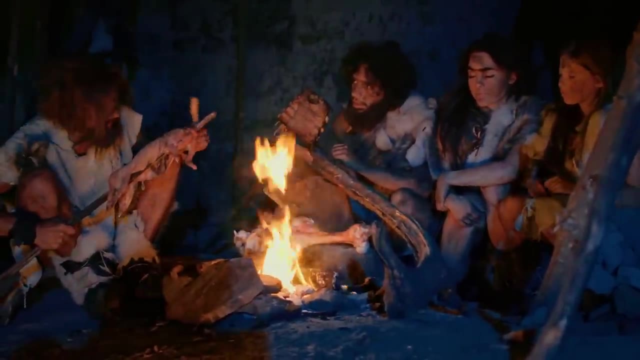 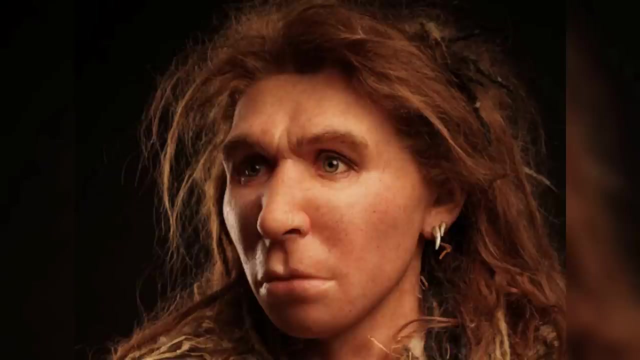 with interbreeding playing a crucial but complex role. Genetic dilution, competitive displacement and the exchange of pathogens are all plausible contributors to their decline. The interbreeding between Neanderthals and modern humans signifies an intricate and pivotal chapter in human history. 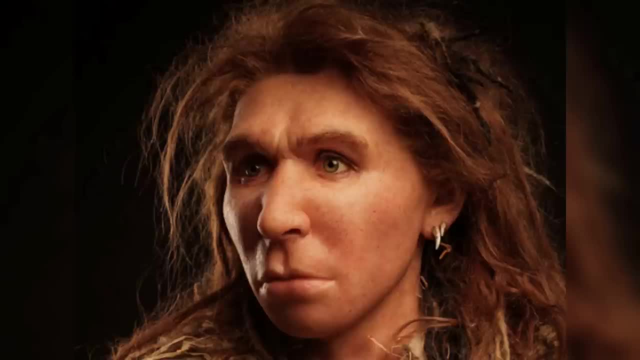 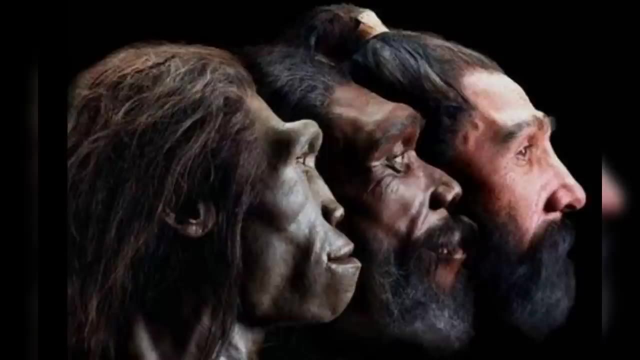 one that continues to be unraveled through ongoing research and discoveries in genetics and archaeology. The misconceptions about Neanderthals being brutish, stooped or hunched have been thoroughly debunked over the years through a combination of archaeological findings. 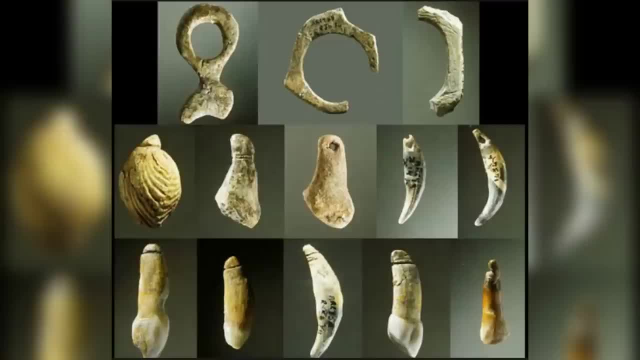 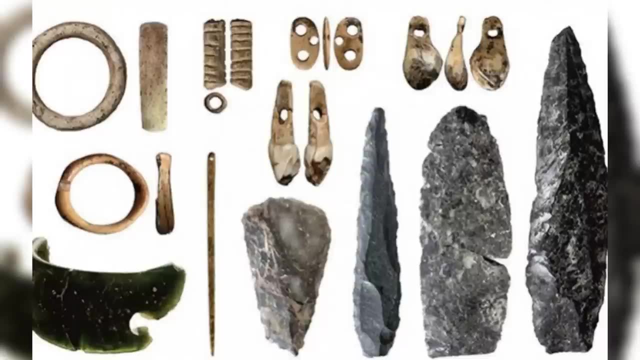 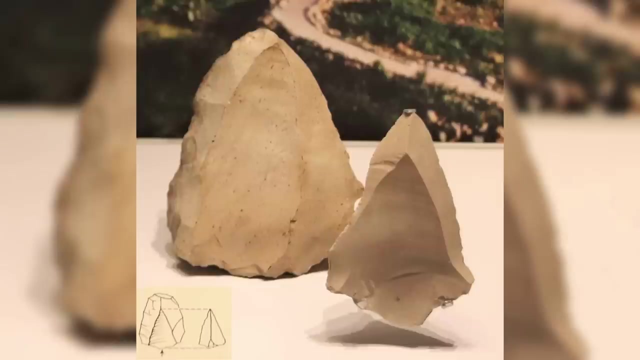 skeletal analysis and genetic research. These studies have painted a more accurate picture of the Neanderthal gene. The image of Neanderthals as primitive brutes was challenged by discoveries of their tool-making abilities, The Mysterian tool culture associated with Neanderthals. 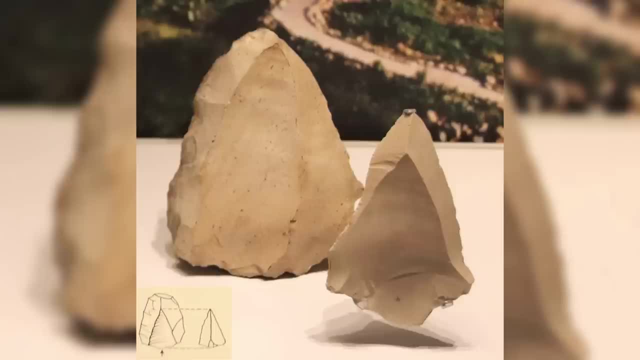 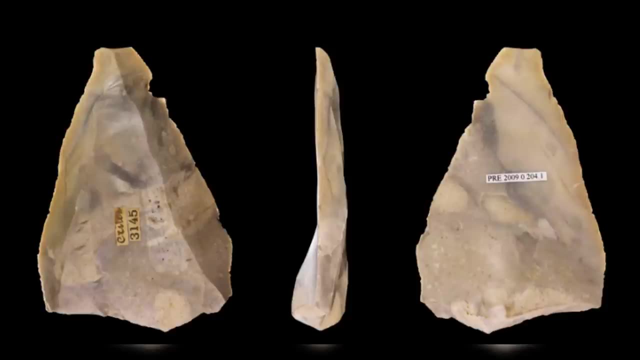 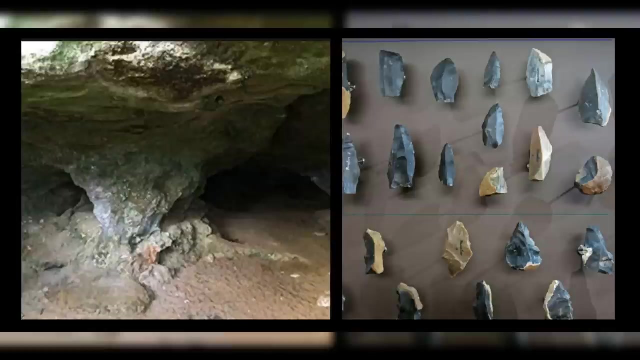 showcased a range of specialized tools made with the Levalois technique. This technique, involving the preparation of a stone core to produce uniform flakes, indicated a high level of planning and creativity- cognitive ability. Sites like Le Moustier in France provided crucial evidence for this. 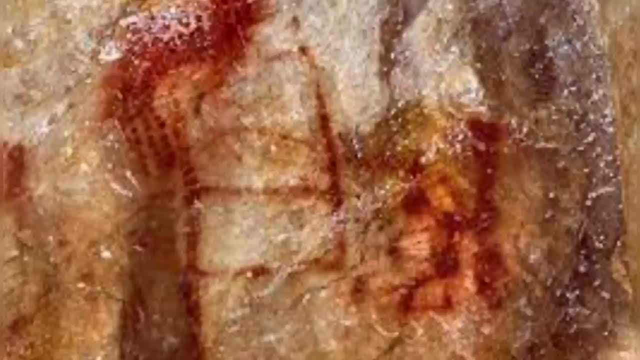 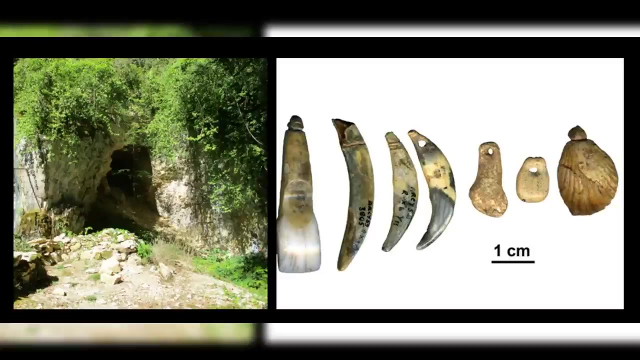 The finding of cave paintings in Spain, such as those in El Castillo, which predate the arrival of modern Homo sapiens in Europe, suggests that Neanderthals engaged in artistic expression. Additionally, ornaments found in sites like the Grotte de Rennes in France indicate a sense of 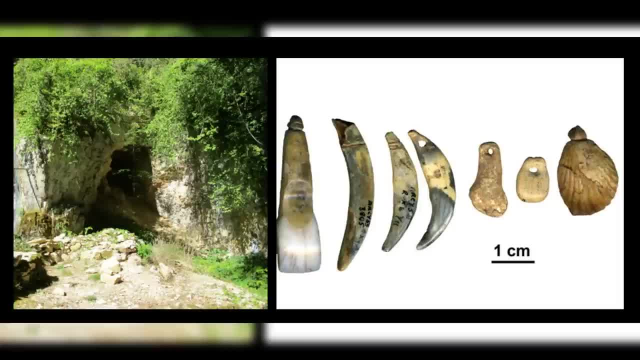 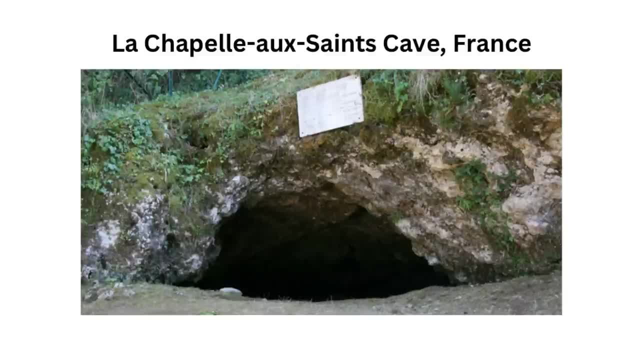 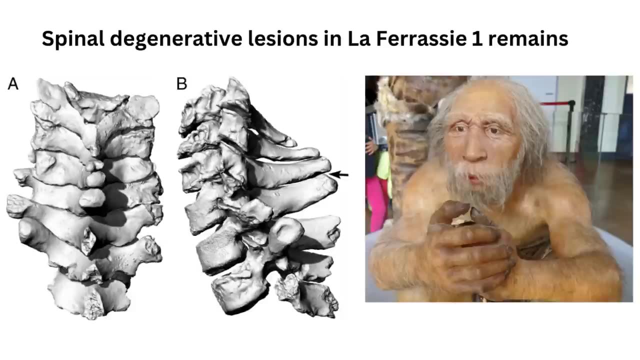 personal adornment and possibly symbolic thought. The misconception of Neanderthals being stooped or hunched originated from an early 20th century analysis of a skeleton found in La Chapelle au Saint, France. The individual was actually arthritic, leading to the incorrect assumption. 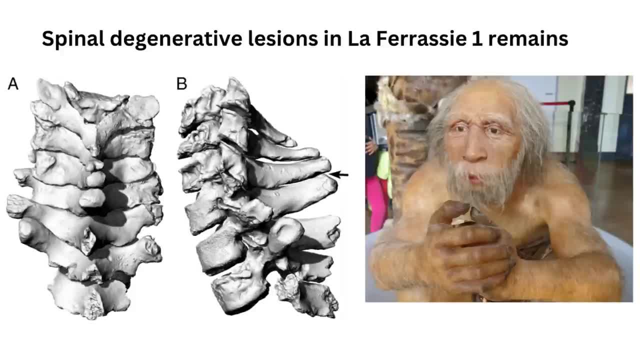 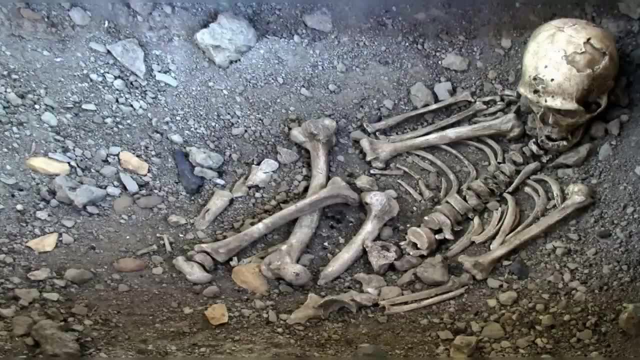 that all Neanderthals had a stooped posture. Later analyses of Neanderthal skeletons showed that their posture was different from that of Neanderthals. Their posture was similar to that of modern humans. Further studies of Neanderthal vertebrae. 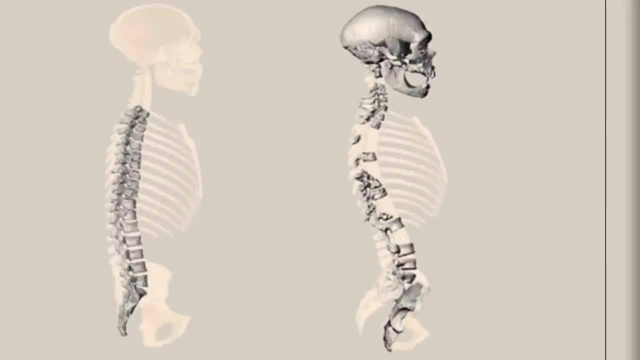 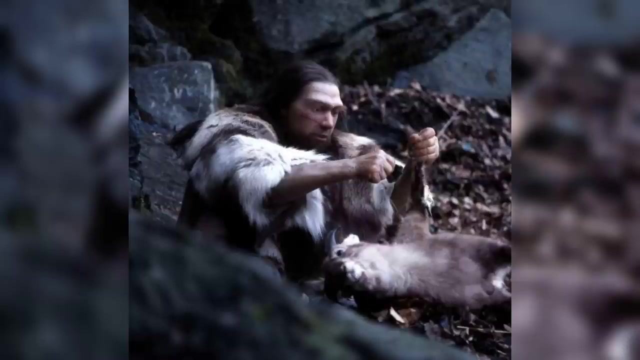 and skeletal structure, such as those conducted by researchers at the American Museum of Natural History, have shown that Neanderthals had a spine similar to modern humans. Their build was robust, adapted for the harsh climates they lived in, but not hunched. 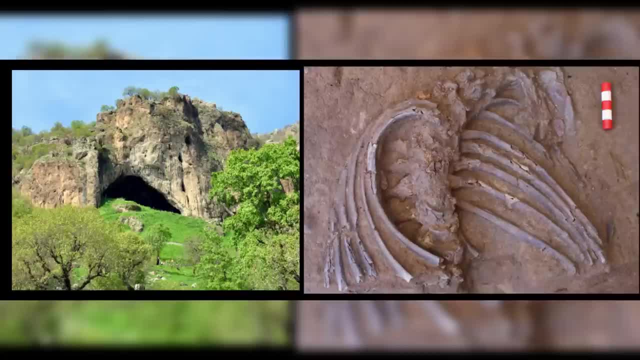 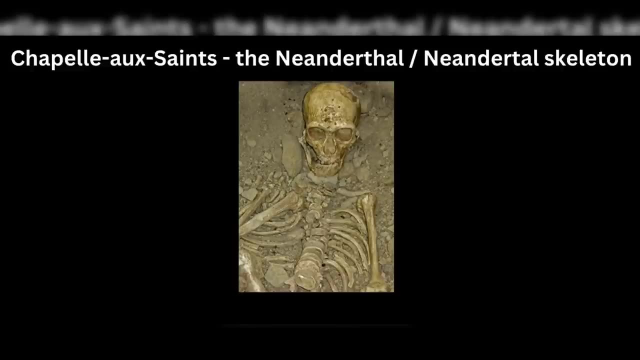 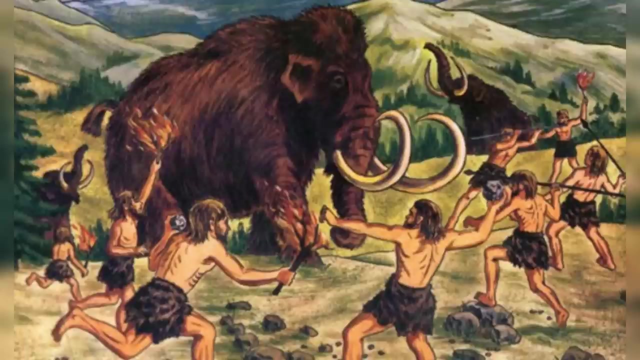 Research on Neanderthal burial sites like those at Shanidar Cave in Iraq suggests that they had complex social structures and possibly even ritualistic practices. The care given to the dead indicates a level of social and emotional complexity not previously attributed to them. Isotopic analyses of Neanderthal remains have revealed: a varied diet, including meat obtained through skilled hunting techniques. This contradicts the notion of them being mere scavengers and highlights their ability to hunt. The sequencing of the Neanderthal genome provided definitive proof of their close relationship to modern humans. Studies led by researchers like Svante Paebo have shown that. 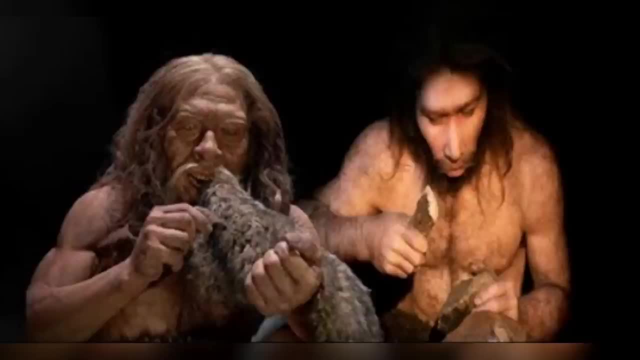 modern non-African humans share a significant amount of DNA with Neanderthals, further dispelling notions of Neanderthals being a vastly inferior or separate species. Genetic research has also suggested that Neanderthals had a similar capacity to hunt. Neanderthals had a similar capacity to 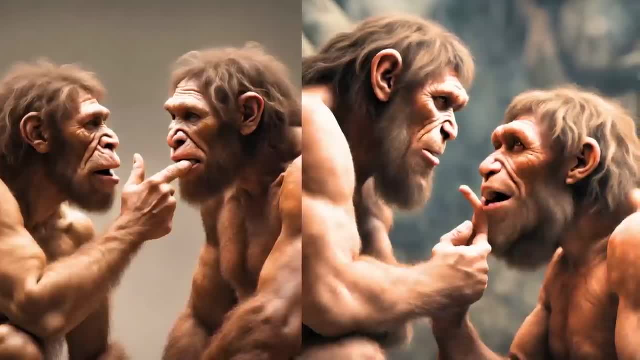 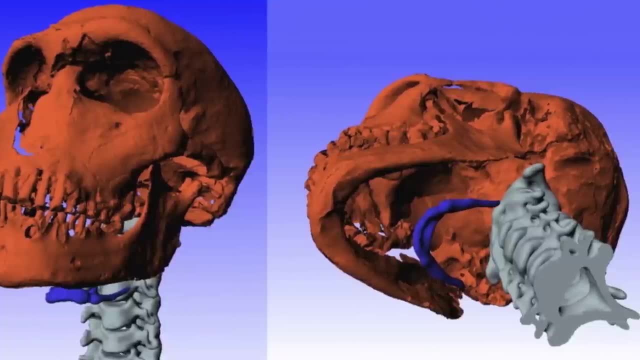 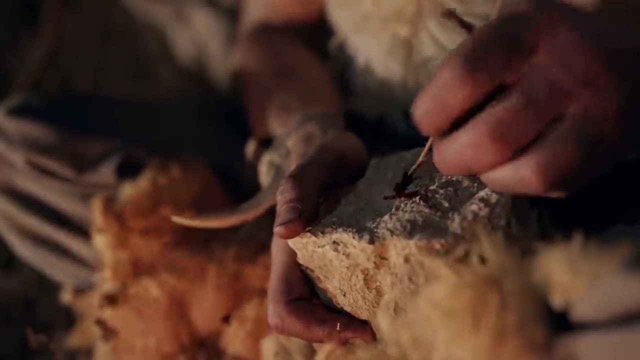 hunt. The discovery of the hyoid bone in Neanderthal remains A bone crucial for speech supported this theory. The image of Neanderthals as brutish, stooped and primitive has been thoroughly revised in light of modern research, Archaeological, skeletal and genetic studies. 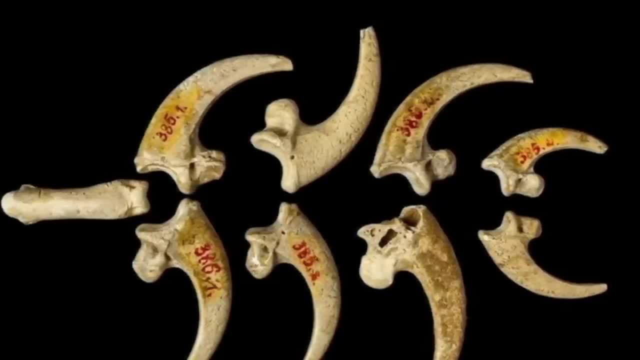 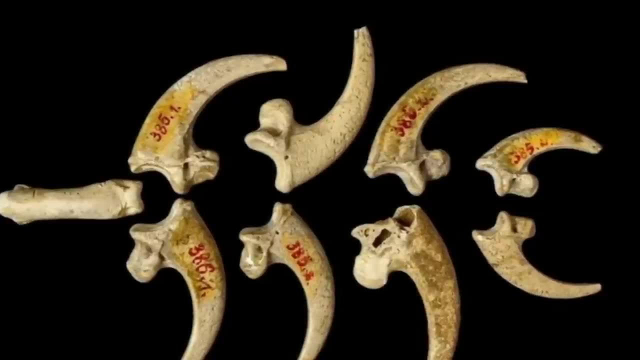 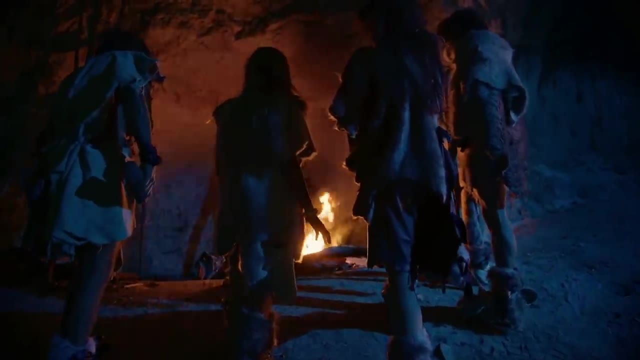 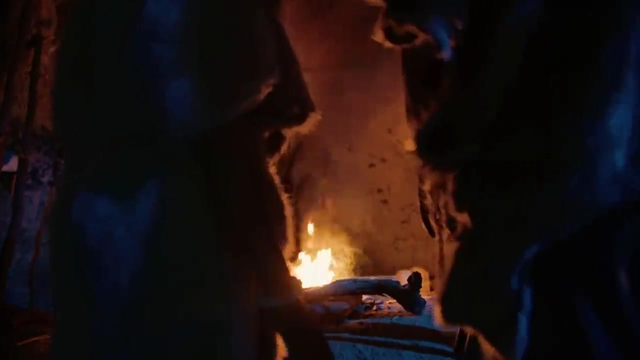 have collectively contributed to a more nuanced understanding of Neanderthals as a complex, intelligent species with many similarities to modern humans. This shift in perception underscores the evolving nature of our understanding of human history and the importance of scientific inquiry in challenging long-held misconceptions. The impact of Neanderthal. 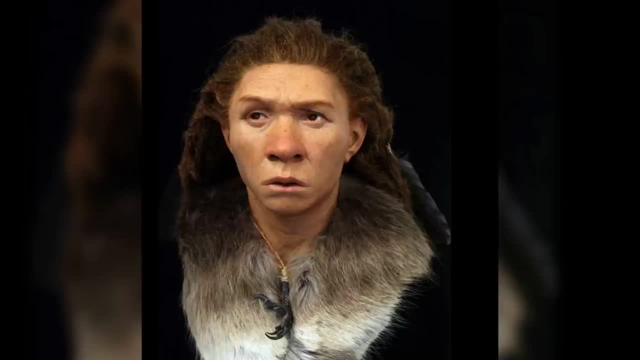 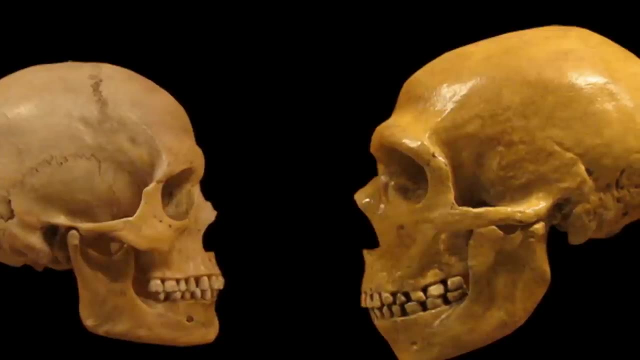 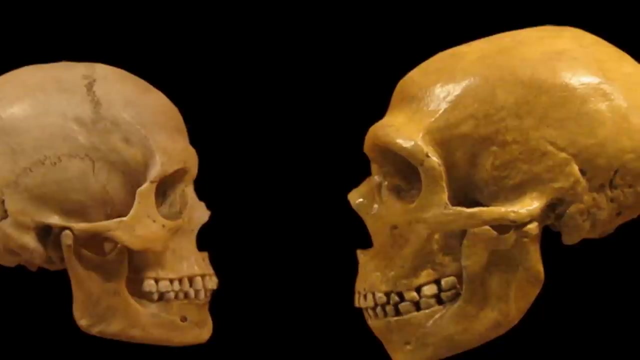 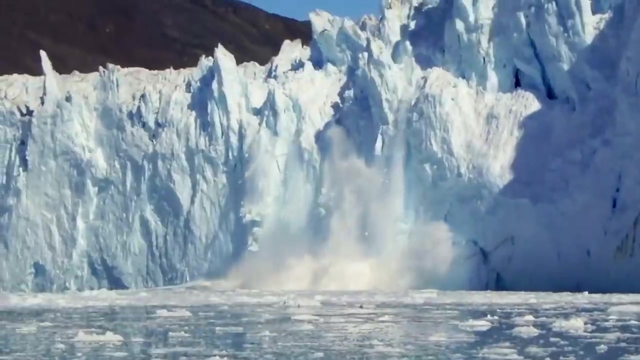 DNA on future human evolution is another topic of ongoing research and interest in the scientific community. While the full implications are yet to be discovered, the study of Neanderthals has not yet been completely understood. Several studies and theoretical explorations suggest various ways in which Neanderthal genetics might influence the growth trajectory of Homo sapiens. 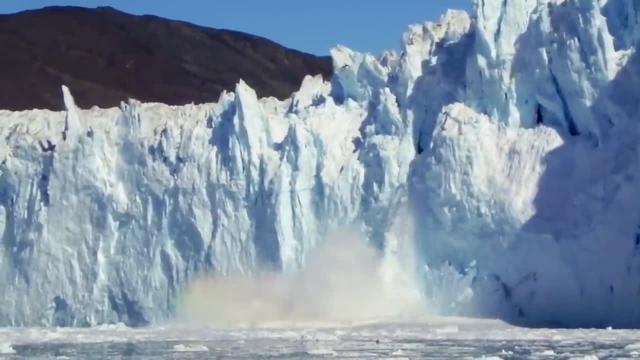 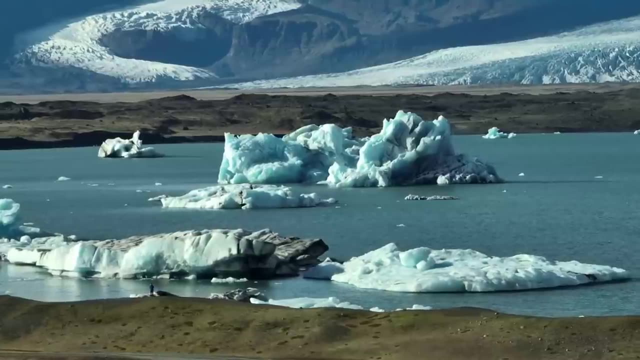 Researchers are exploring how Neanderthal genes related to physical adaptations might influence human resilience in the face of climate change. Given that Neanderthals survived harsh fluctuating climates, genes related to human resilience might also influence human resilience in the face of climate change. 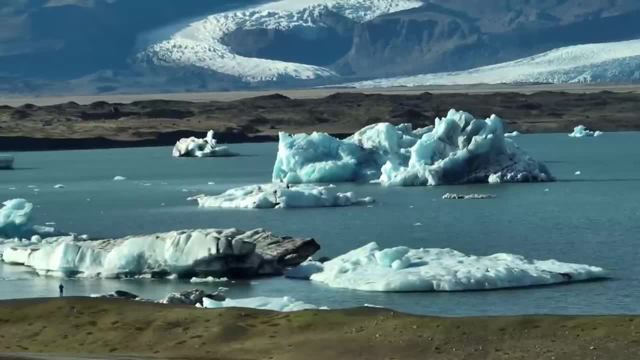 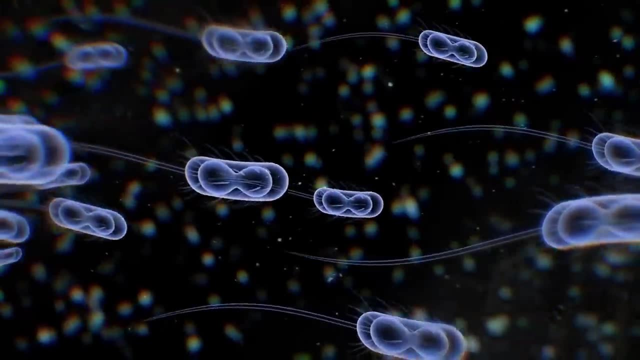 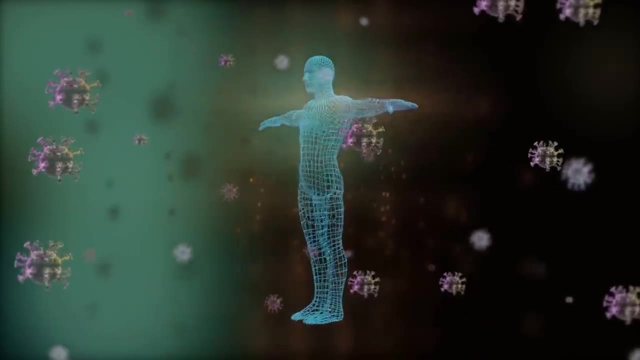 Neanderthal genes related to cold tolerance and metabolic efficiency might become advantageous as humans face new environmental challenges. Studies have shown that some Neanderthal alleles contribute to the modern human immune system. As global health challenges evolve, these genetic traits might play a role in human 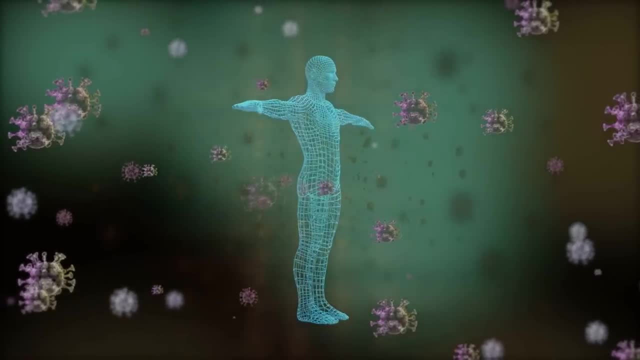 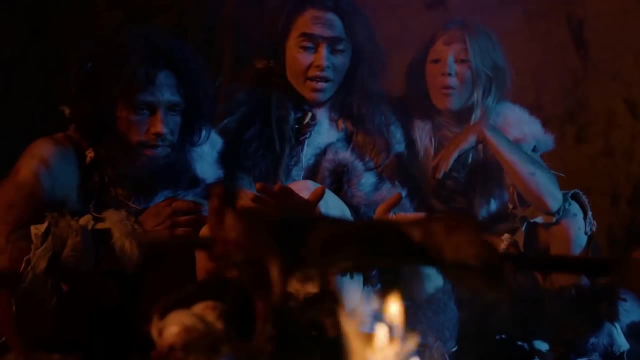 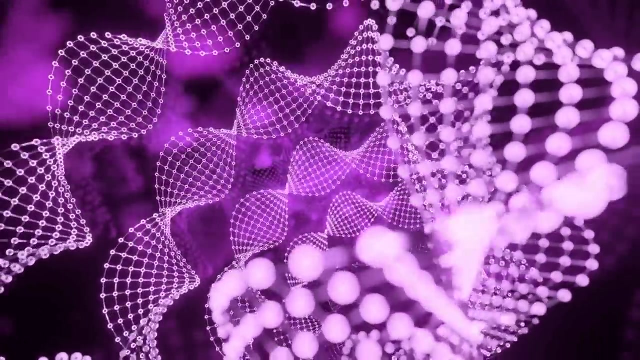 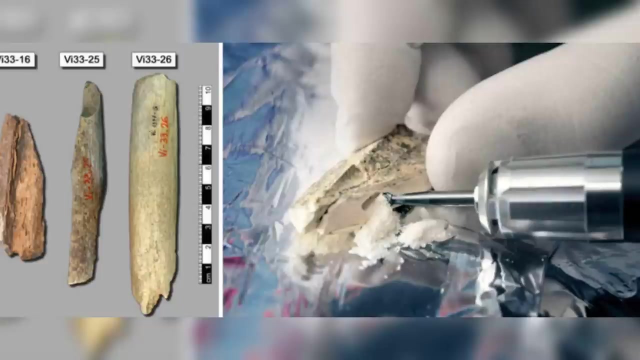 populations' ability to resist or adapt to new diseases and pathogens. Ongoing research, including that by the Stanford University School of Medicine, is examining the relevance of these genes in contemporary health contexts. The genetic contribution from Neanderthals has added to the overall genetic diversity of the human population. 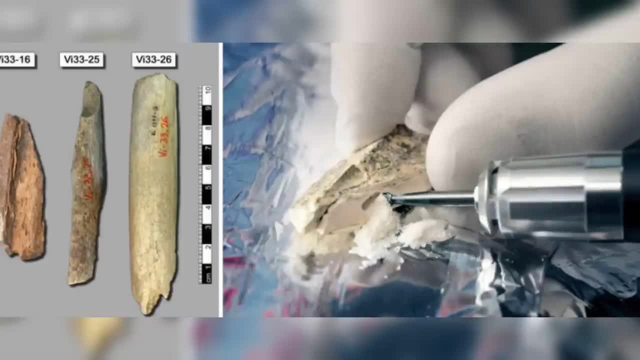 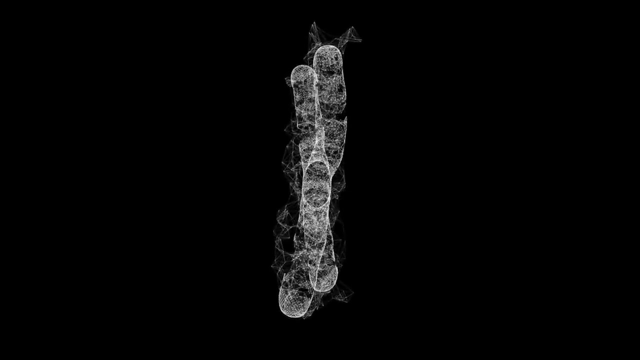 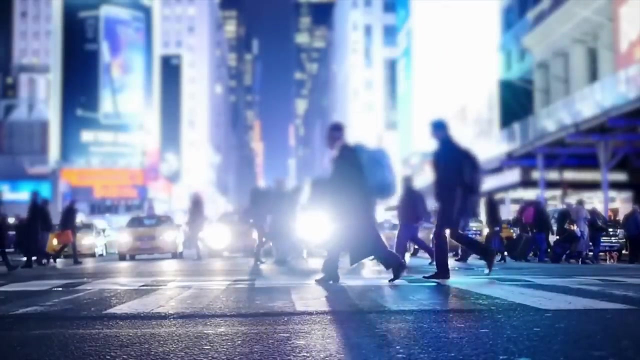 Researchers, including those at the Max Planck Institute for Evolutionary Anthropology, are studying how this diversity might affect human adaptability and resilience, potentially influencing growth processes. Genetic studies are also considering how Neanderthal alleles might influence aspects of human development and reproduction. Variations in fertility, gestation and developmental 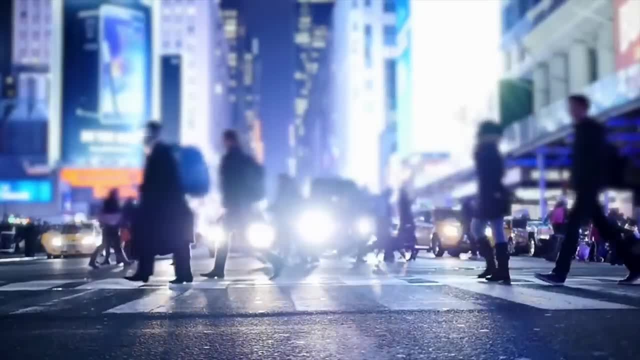 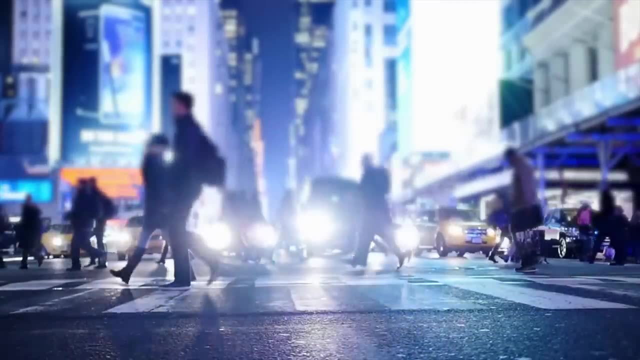 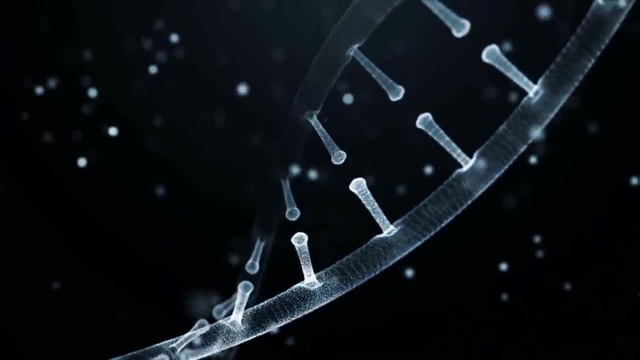 processes influenced by these ancient genes could subtly impact the future demographic patterns and growth trajectories of human populations. As humans continue to develop alongside rapidly advancing technologies, we will continue to see that the role of ancient genetic traits in this interaction is a subject of interest. 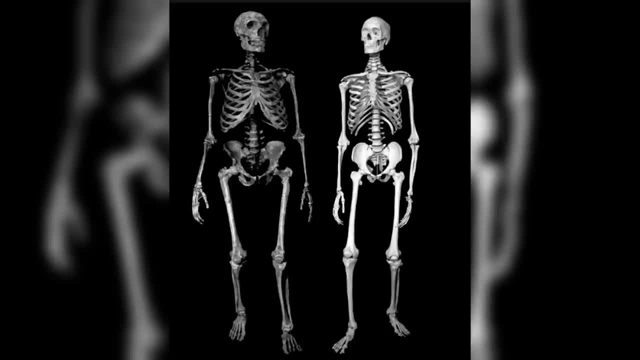 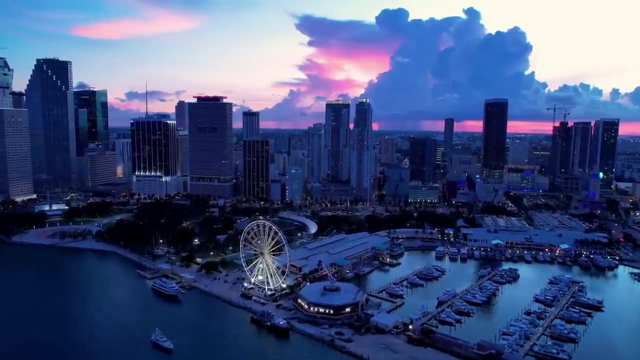 The integration of technology in healthcare and daily life may interact with genetic predispositions, including those from Neanderthal heritage, in ways that could shape future human development. Modern lifestyles, particularly in urban settings, present new environmental and health challenges. Ongoing research is looking into how inherited 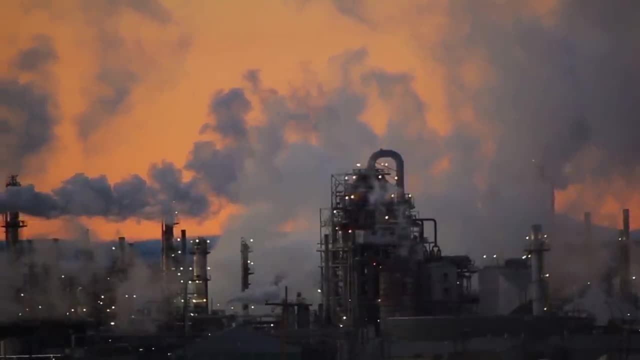 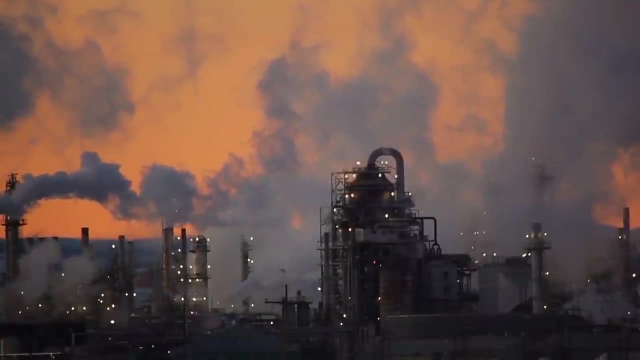 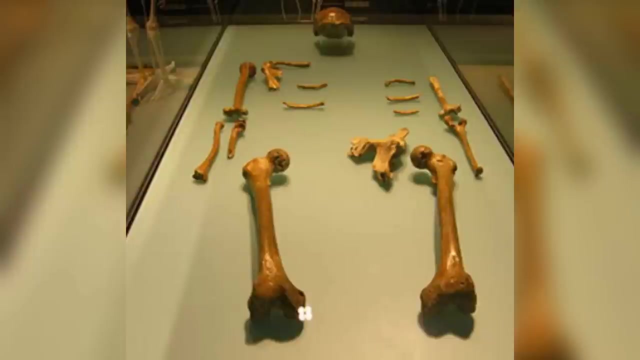 Neanderthal traits affect human development. Neanderthal traits have been identified as natural andácritic issues or, specifically, threat from ancestral diseases or biologicalרגibility. Moreover, the use of genetic studies may concern the ability of humans to adapt to these new environments, considering factors like pollution, dietary changes and sedentary lifestyles. The study of Neanderthal DNA's impact on future human evolution is increasingly interdisciplinary, involving collaborations between geneticists, anthropologists, climate scientists and medical multifaceted ways in which ancient genetics might interact with modern and future environments. 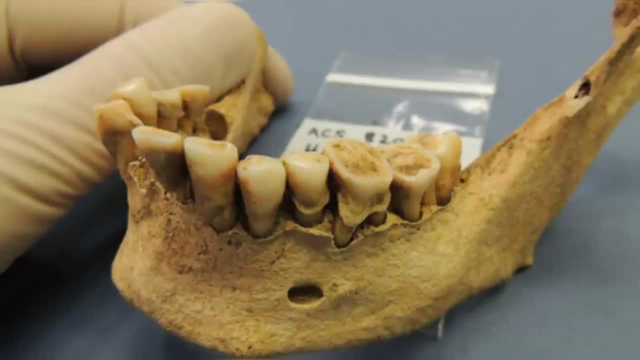 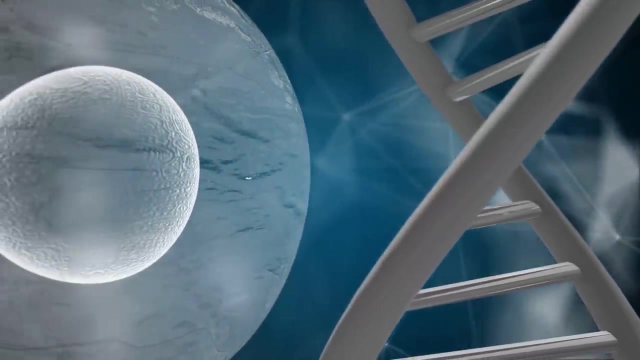 As research progresses, it continues to shed light on how these ancient genetic influences might shape human adaptability, health and resilience in an ever-changing world. Understanding our genetic history, particularly in the context of Neanderthal DNA and its integration into the modern human genome, is crucial for several reasons. 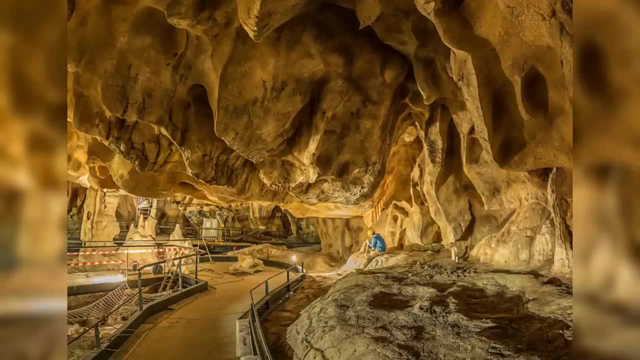 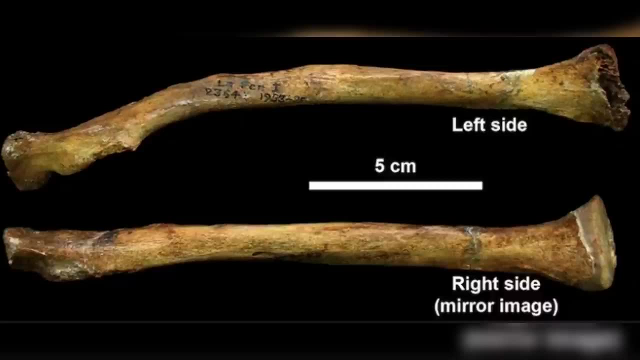 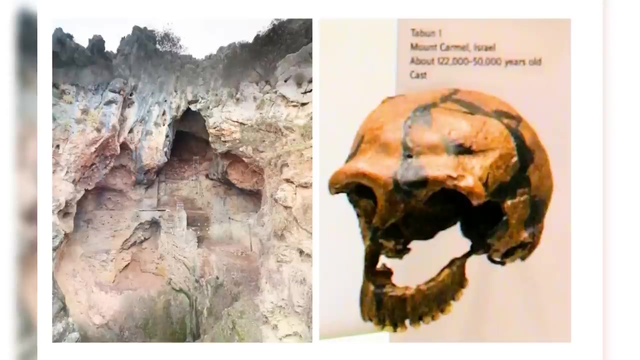 It sheds light on our past, influences our present identity and potentially guides our future as a species. The discovery of Neanderthal DNA in modern humans has revolutionized our understanding of human growth. It challenges the simplistic view of a linear evolutionary path and reveals a more complex 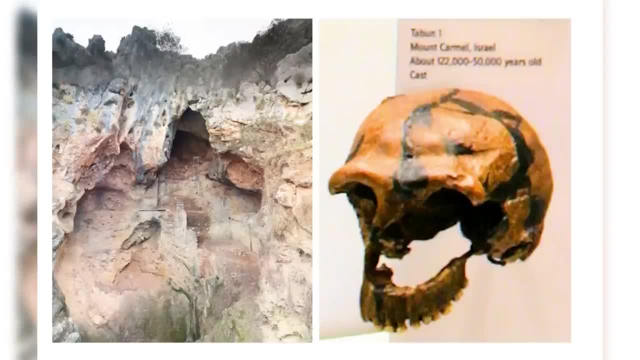 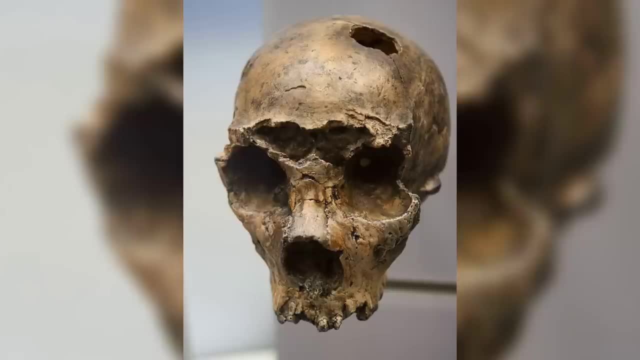 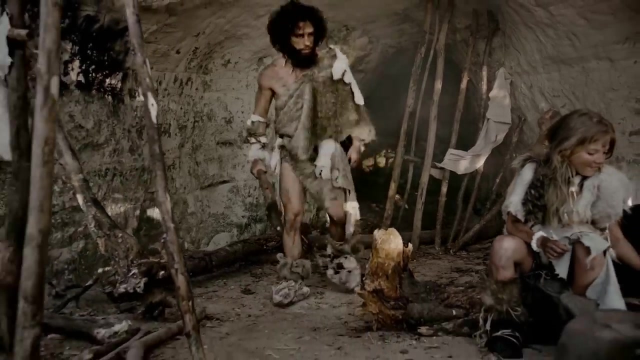 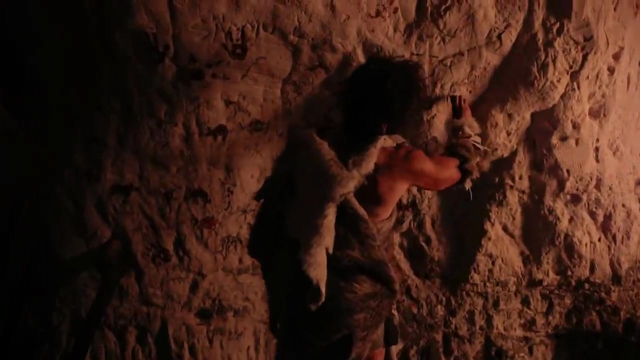 narrative, with multiple hominin species interbreeding and interacting. This complexity highlights the dynamic nature and the myriad factors that shape a species. Understanding our genetic history has led to a re-evaluation of Neanderthals, Once seen as inferior and brutish, the recognition of their genetic contributions to modern humans. 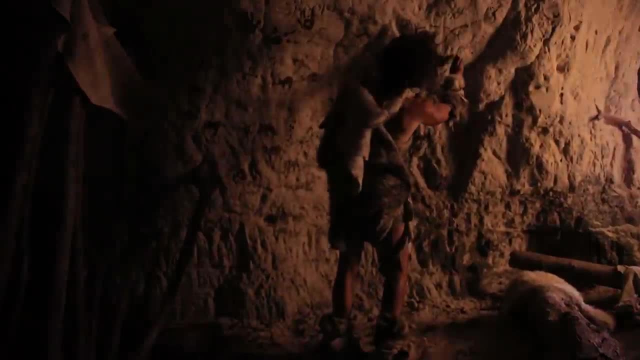 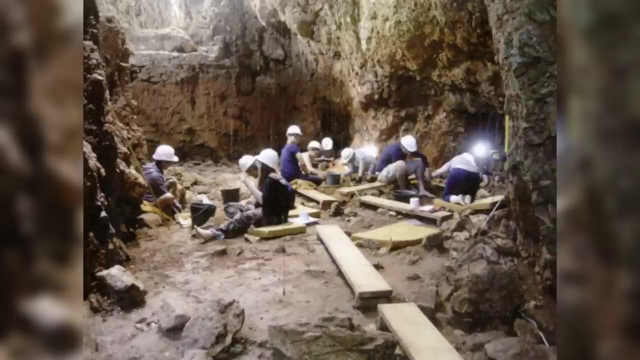 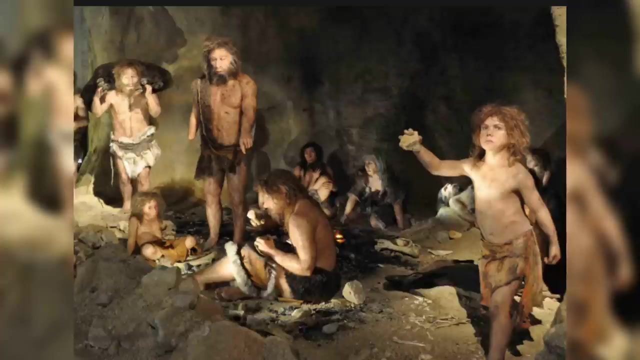 has elevated their status in human history. This shift in perception illustrates how scientific advancements in the history of Neanderthals can re-shape our understanding of history and identity. The genetic legacy we carry influences not just our physical traits, but also aspects of our behaviour, health and perhaps even cultural practices. 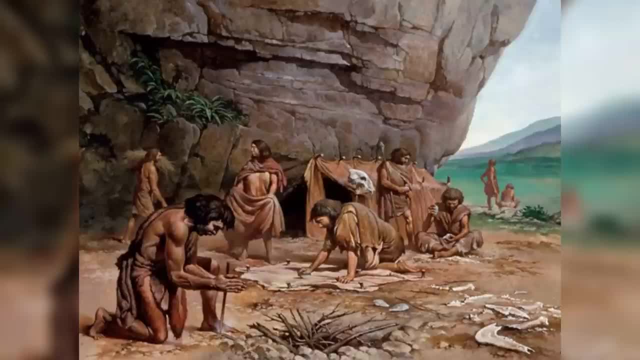 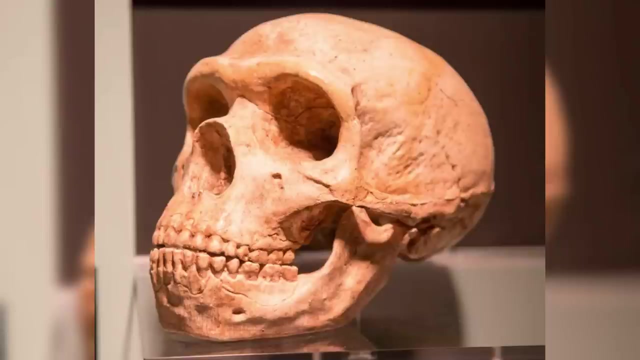 By acknowledging the Neanderthal components within us, we gain a deeper understanding of the biological and cultural threads that contribute to the tapestry of modern human living identity. While there is great diversity within Homo sapiens, our shared genetic history with other hominins like Neanderthals, underscores a fundamental 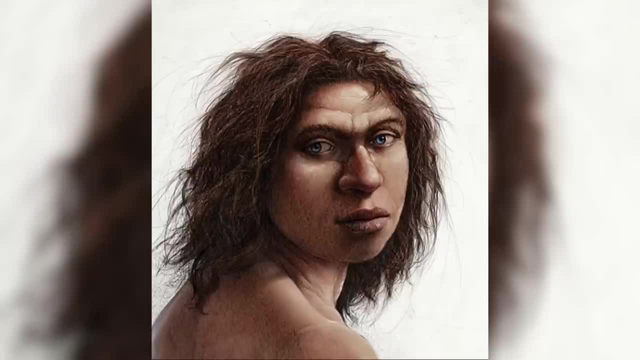 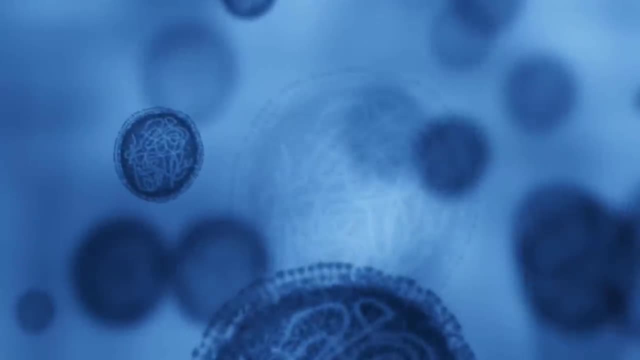 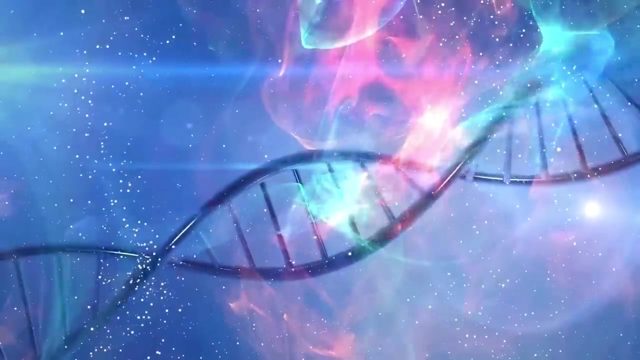 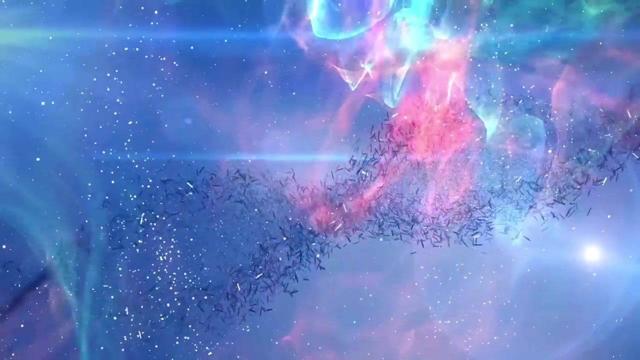 unity. It emphasizes that diversity and adaptation are intrinsic parts of our journey. Neanderthal genetics have practical implications in medicine. Understanding the specific roles of these ancient genes can inform the treatment and prevention of diseases, as well as offer insights into the human body's response to various environmental factors. This knowledge is pivotal in the 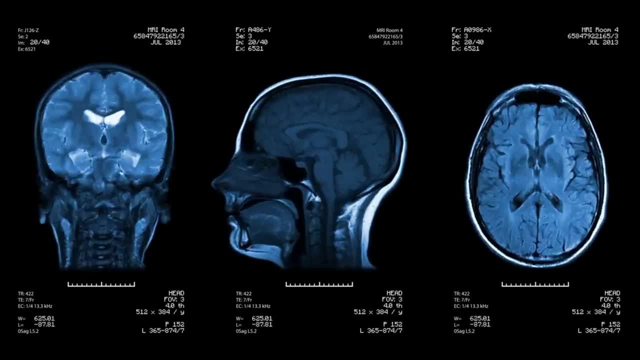 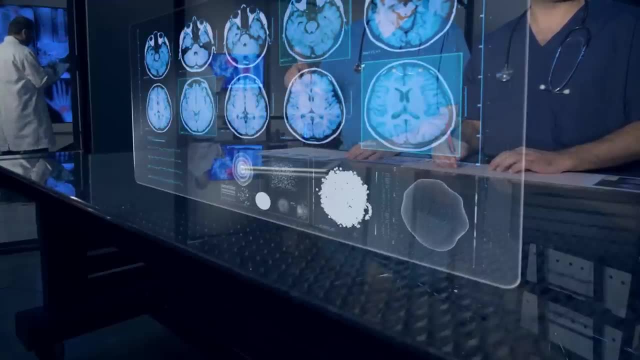 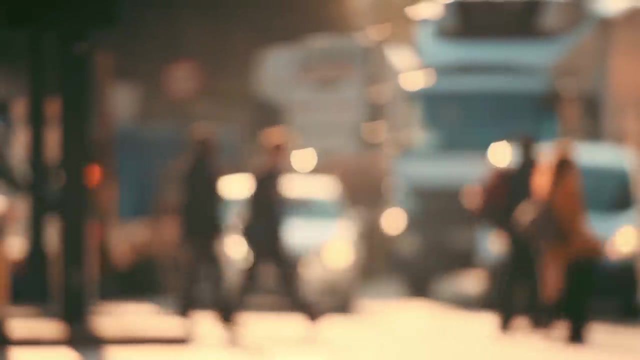 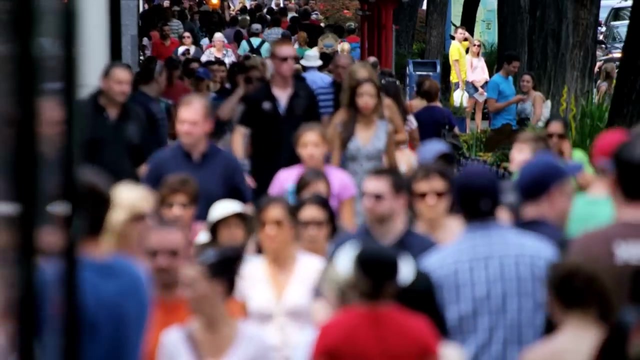 era of personalized medicine and genomic health care. It helps in understanding how past adaptations and interbreedings have shaped our current vulnerability or resistance to genetic change. Our genetic history can offer clues about how humans might adapt to future environmental and societal changes, Understanding past adaptations, especially 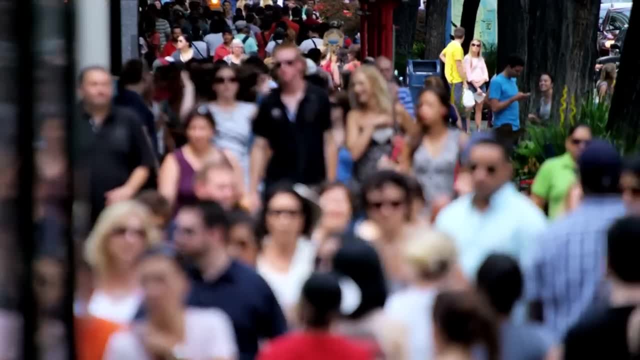 in the face of climate change and global health challenges can inform predictions and preparations for the future. The exploration of our genetic past also allows us to understand the future of our future. The exploration of our genetic past also allows us to understand the future of our. 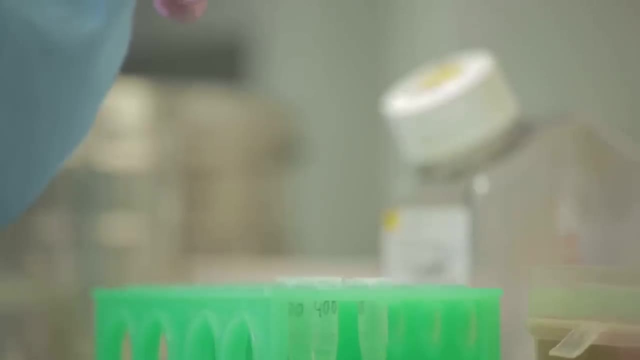 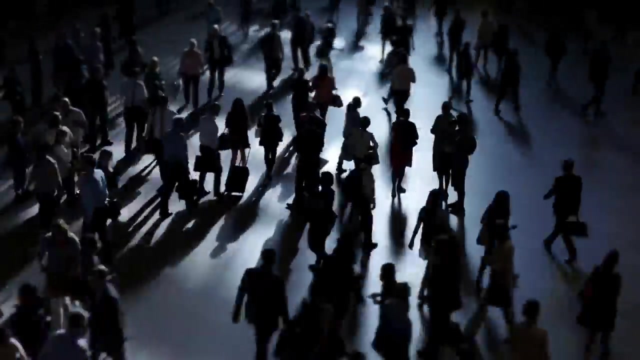 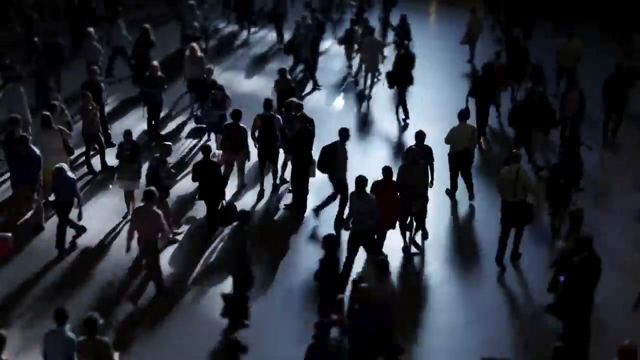 future. The exploration of our genetic past also raises important ethical questions about genetic research and manipulation. It prompts a broader discussion on how we should use our growing understanding of genetics, considering the implications for identity, privacy and the essence of what makes us human. Reflecting on the importance of understanding. 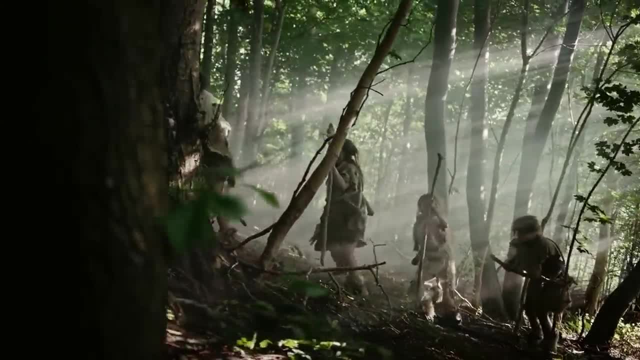